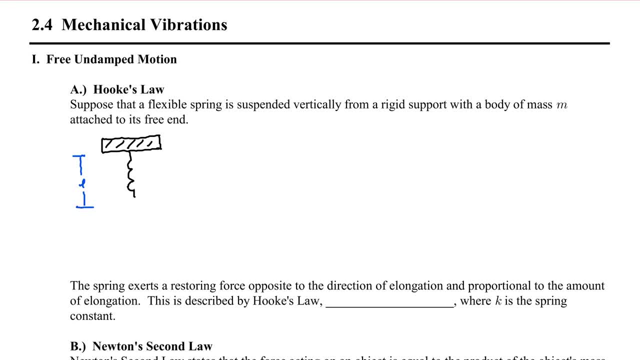 in its unstretched form, is called L. This is the startup of our experiment. This is the unstretched spring. Now, what we're going to do, phase two: here we're going to keep this rigid support, but we're going to take a mass which we'll model with mass m and we're going to attach 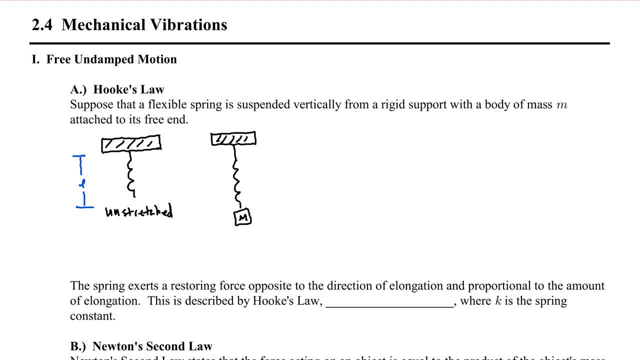 it to the end of that spring. That's going to cause the spring to stretch a little bit. Now, as you can see, we're going to stretch the spring a little bit, but eventually it will come to rest in what we call static equilibrium. Static means it's not moving, it's not isolating Equilibrium. 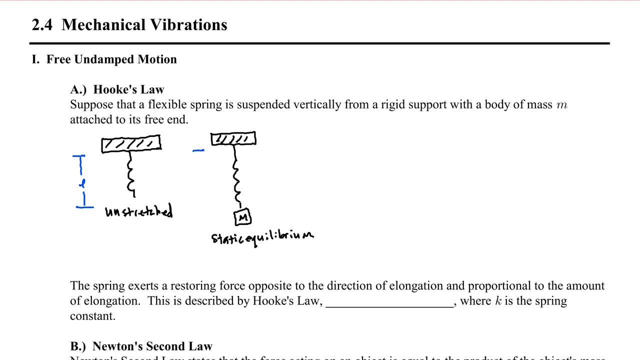 means that it's come to a balanced position. Now, remember the original length of the spring. we designated as L, and when we stretch the, when we hang the mass, it's going to stretch the spring just a little bit. We'll call that distance S naught for static equilibrium. Now, if you saw this set up, 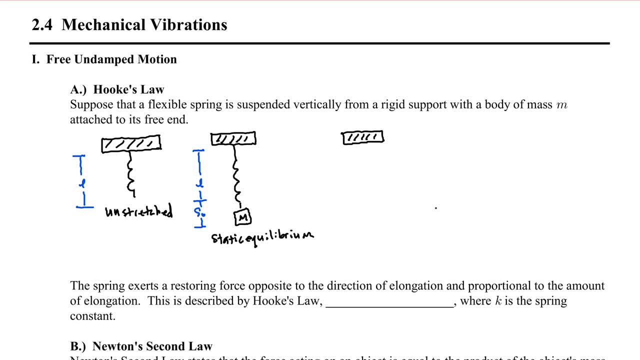 in lab. what would you do with that mass? It'd be irresistible, right? You'd want to reach up and pluck that mass, pull it down and watch it oscillate. So I'm going to assume that I reach up and I pull the mass down and I release it. It's going to oscillate up and down. This is what we. 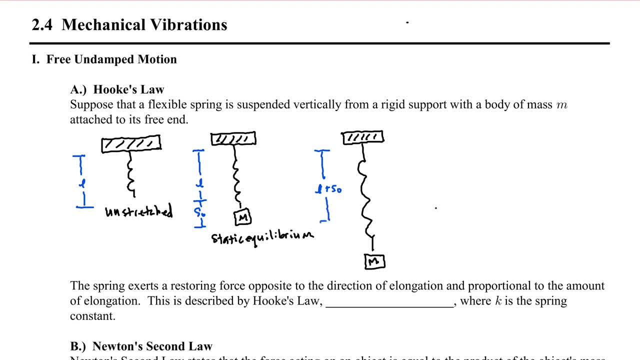 want. So the length of the spring in static equilibrium. now we can model as L plus S, naught, and then the string, the spring has been stretched. We're going to call that distance X. Specifically, X represents the position of the mass. 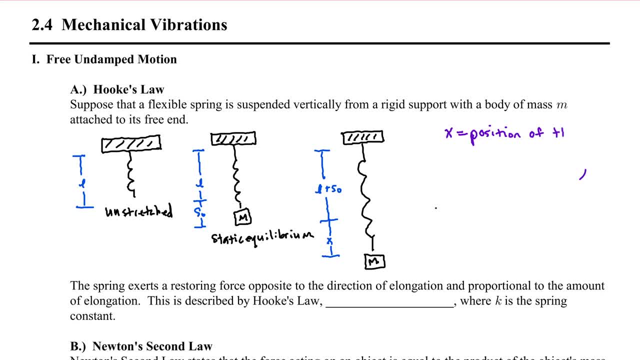 beyond equilibrium, When we recognize that our equilibrium position is here. if we stretch the mass below that equilibrium position, then X is going to be positive. So when X is greater than zero, the mass has actually moved down. So positive X means we have motion in a downward direction. 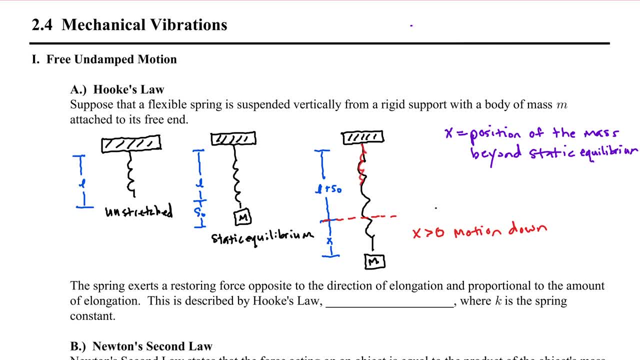 If we compress the spring- let's show another phase here- then the mass has moved up, but the spring has been condensed or compressed. So when X is negative, this is describing motion up. So there's a little bit of a disconnect there. You've got to remember that when you construct your models. 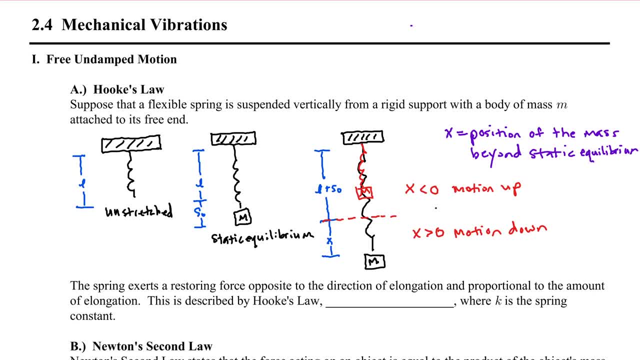 that a negative position is above equilibrium and a positive position is below equilibrium. Both Hooke's law and Newton's second law will govern the long-term motion of this spring Before the mass is set in motion. when it's in static equilibrium, we can observe that the weight 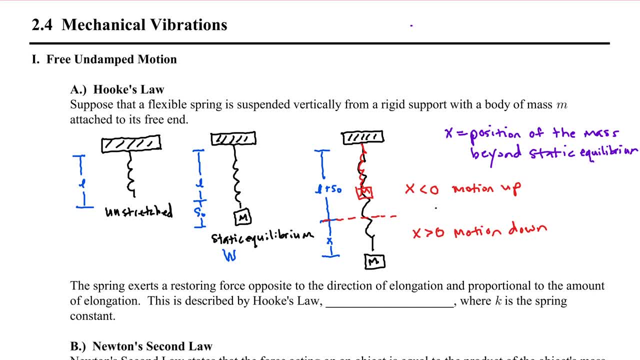 of that mass. remember weight and mass are different. the weight of the mass is equal to the restoring force of the spring. So static equilibrium once again means there's no motion. But when plucked the spring will exert a restoring force opposite to the direction of. 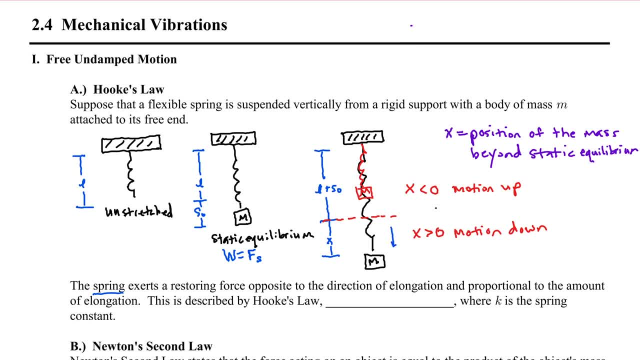 elongation. So if I pull the mass downward, the spring is going to want to get back to that static equilibrium position, So it's going to exert a force in the opposite direction. Or if we compress the mass upward, the spring will exert a restoring force in the opposite direction, always longing to 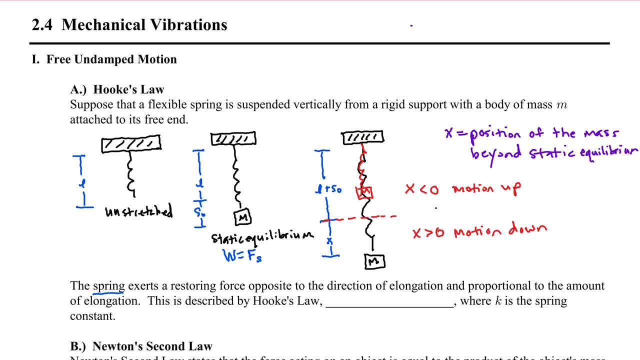 get back to that static equilibrium position. In particular it is proportional to the amount of elongation. So this is described by Hooke's law: The force in the spring is equal to negative k times x, where k is the spring constant. 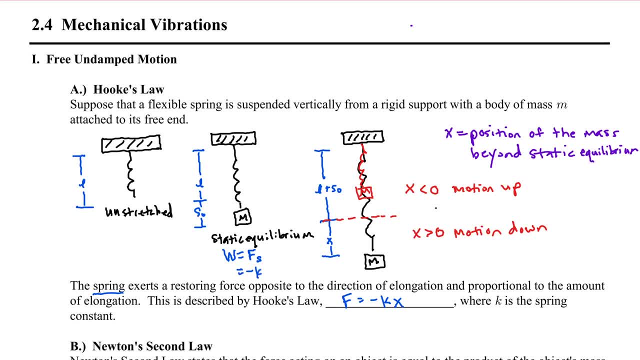 So if the force of the spring is given by Hooke's law as negative kx and it's in the opposite direction of the weight, weight is calculated as mass times gravity or mass times acceleration, which is the force of the spring. So if the force of the spring is given by Hooke's law as negative, 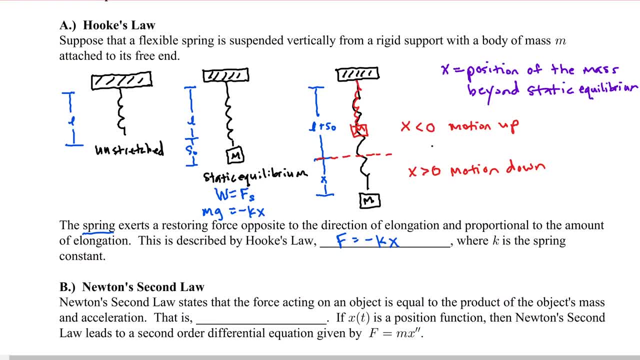 kx, which is what Newton's second law is all about. Newton's second law states that the force acting on an object is equal to the product of the object's mass and acceleration. That is, force equals mass times acceleration. In our example here we've expressed acceleration as the acceleration of gravity. 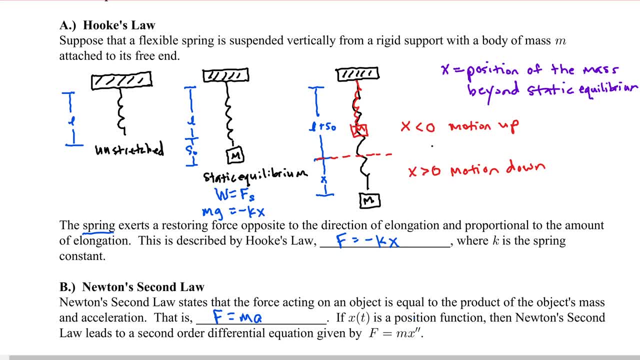 If x of t is a position function, so we're modeling the position of the mass at times t, then Newton's second law leads to a second order differential equation given by f equals mx double prime. So mass times acceleration can now be modeled by m times x double prime. 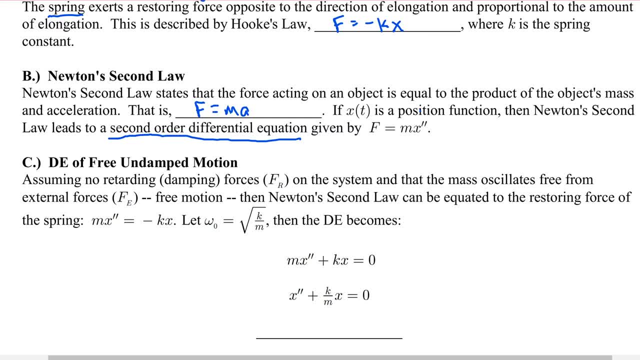 When we combine Hooke's law and Newton's second law, we can generate a differential equation of free- undamped motion. Now we're qualifying this motion as both free and undamped, and we'll vary that as we increase the complexity of our experiment. Free simply means that there is no external forces. 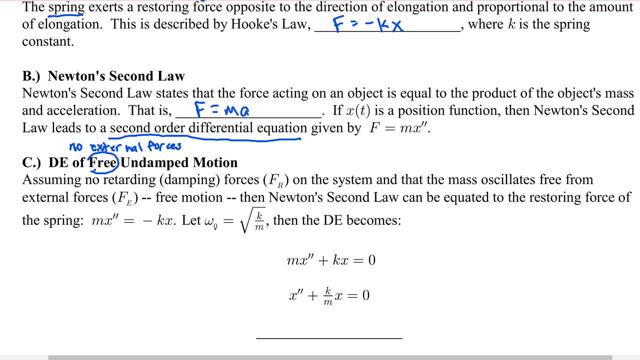 acting on this object. For example, if I were to interfere with that rigid base, maybe move it up and down, then we would call that driven motion. So we're studying free motion to begin with. Also, this is undamped motion. 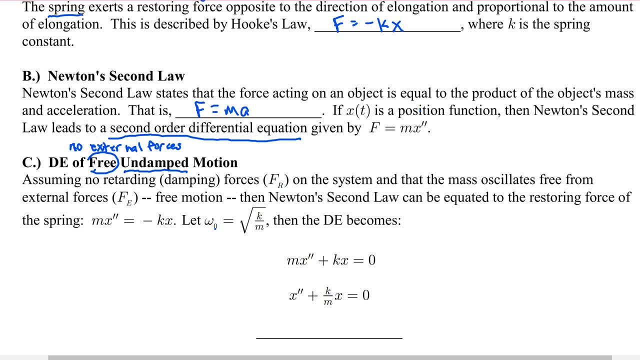 So there's no resistance to the velocity of that mass. That is. undamped motion simply means that there is no impedance to the motion, There's no deceleration, no shock absorbers or anything like that. So this is the simplest possible case: Free, no external forces acting on this setup and undamped motion. 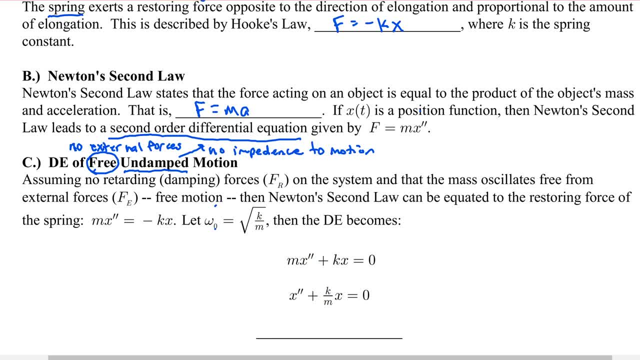 That means there's no impedance to the motion, Assuming no retarding or damping forces F sub r on the system and that the mass oscillates free from external forces. this is free motion. then Newton's second law can be equated to the restoring force of the spring. 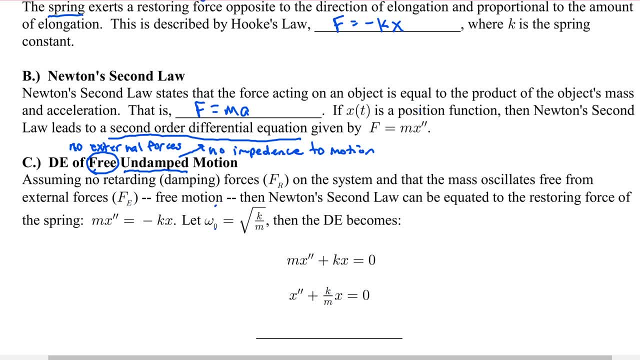 That is m x, double prime. that means mass times. acceleration is equal to negative k x, and that comes of course from Hooke's law. So, starting with this balanced equation, we can add the term k x to both sides. 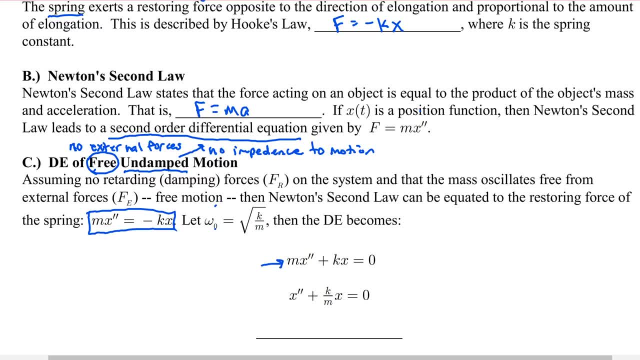 and what we observe here is that we have a linear, second order, homogeneous differential equation with constant coefficients, And this is the exact type of equation that we've been studying how to solve. This is what we call the differential equation of free, undamped motion. 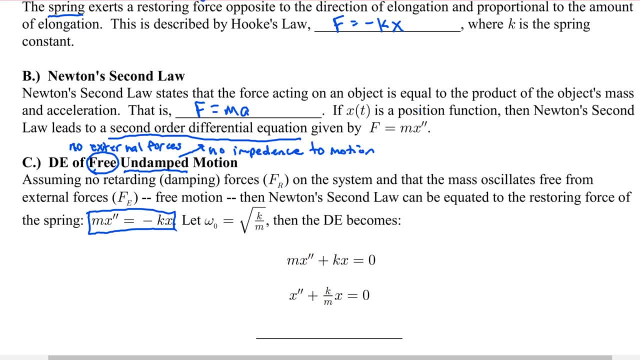 Now, in order to analyze certain situations and solve this in general, we're going to manipulate the coefficients to make our analysis a little bit easier later on. this constant called omega naught, Let omega naught equal the square root of k over m At this. 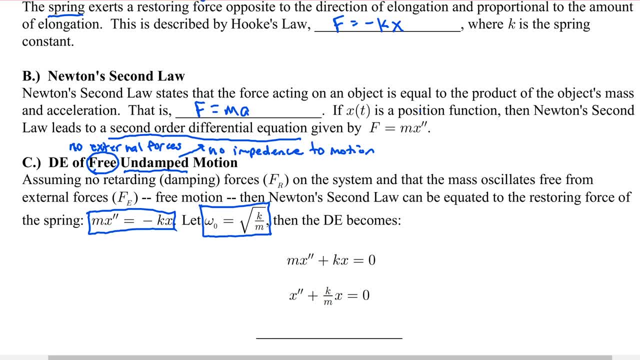 point. it doesn't make any sense why we did that. but again, when we get to the general analysis here in a minute, you'll see this is going to simplify some of our notation. So back to our d? e of free, undamped motion. I'm going to start by dividing all three of those terms by m, So we have x double. 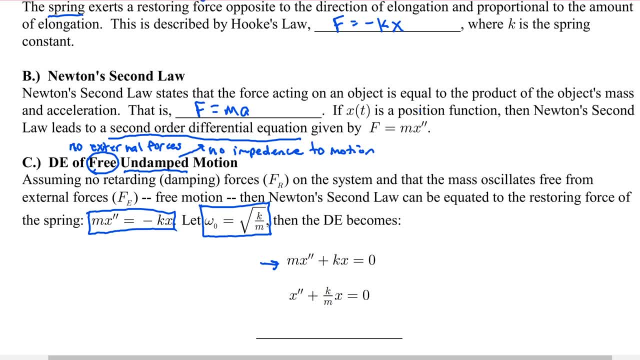 prime plus k over m times x equals zero. Then we see this coefficient k over m and we have defined omega naught to be the square root of k over m. So we could rewrite this differential equation as: x double prime plus omega naught squared times x equals zero. So the original equation and this: 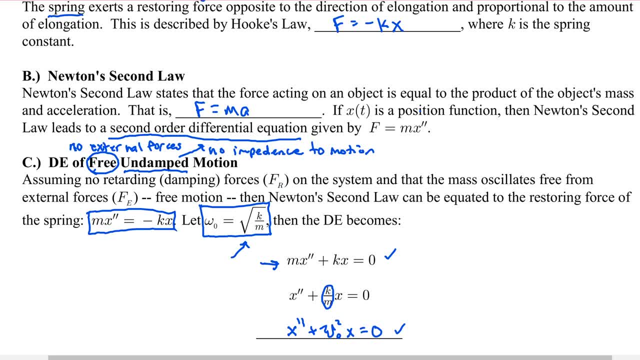 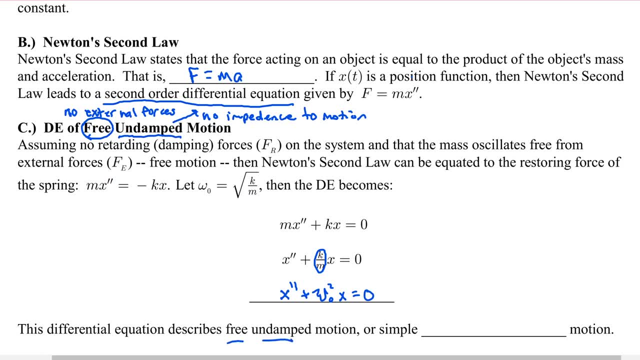 one are equivalent. We've just manipulated the coefficients for simplicity later on. This differential equation describes free undamped motion, also known as simple harmonic motion. That is, the spring or the mass will oscillate above and below the equilibrium position indefinitely. Remember, later on we will program into our differential equation damping. 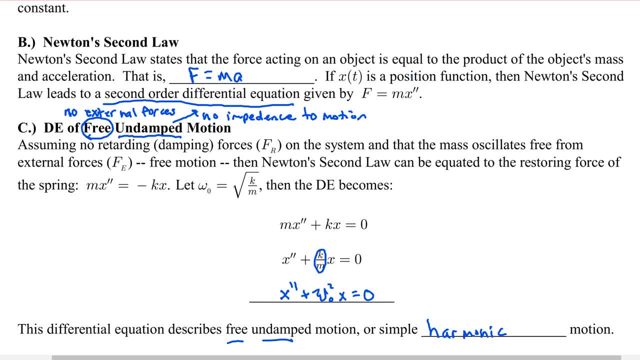 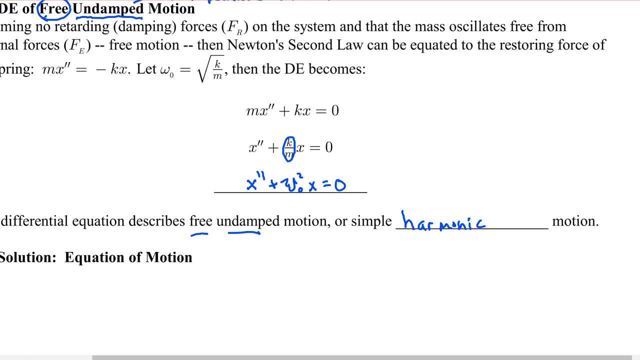 forces such as air resistance or some sort of shock absorber. Right now, we're just getting started with our differential equation, So we're going to start by dividing all three of these with simple harmonic motion. Now our next goal is to solve this differential equation in general. 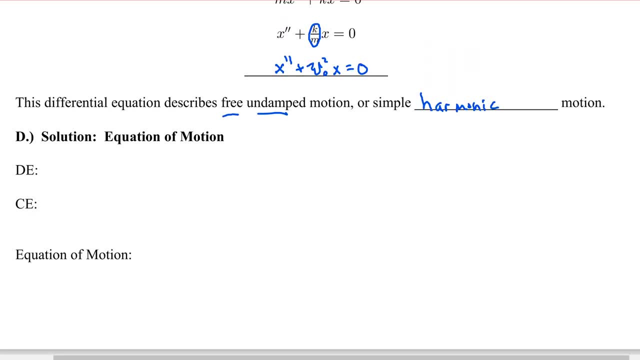 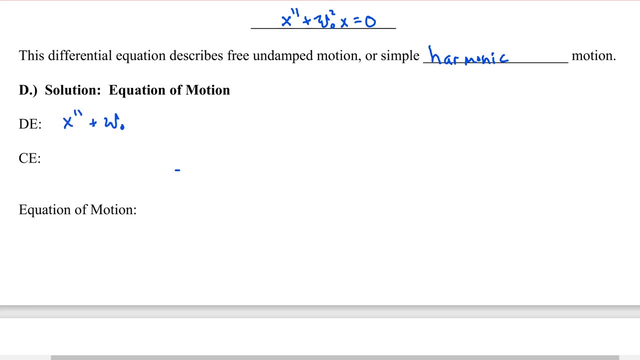 This is why you'll see that we introduce that constant omega naught squared, Starting with our differential equation. x double prime plus omega naught squared x equals zero. The corresponding characteristic equation would be: r squared plus omega naught squared, equal to zero. If we solve this equation for the roots, r squared would be negative omega naught squared, and if I 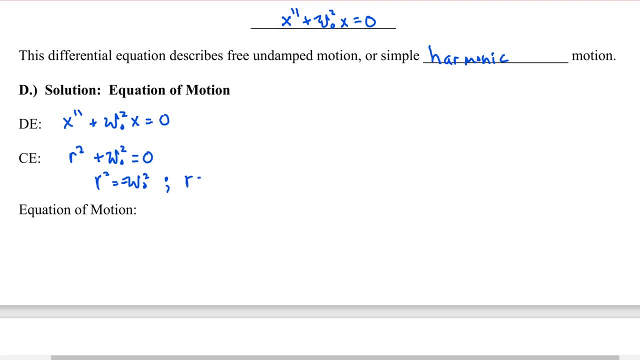 take the square root of both sides, that's going to give me r equals plus or minus omega naught. i. So, again, a moment ago we said omega naught equals the square root of k over m, so that we could get an omega naught squared here. and what's the purpose of that? Well, now, when I take the square, 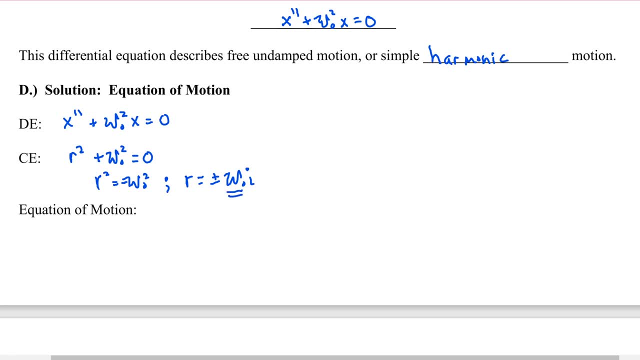 root of both sides. I have this very simple constant to deal with. Remember it was negative. so we do have here two distinct imaginary or complex conjugate solutions. Because of the nature of the roots, of the characteristic equation, we can then derive our equation of motion or the solution to 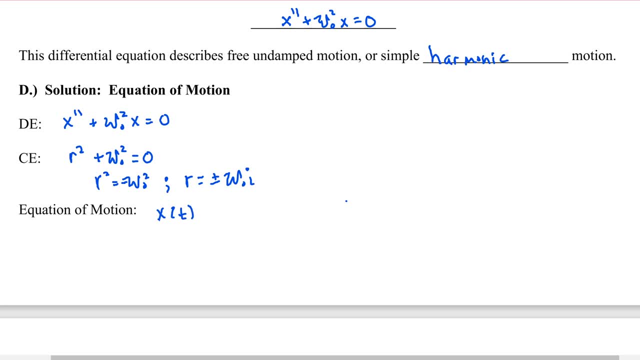 this differential equation, Our solution, dependent variable x, independent variable t- would be e to the zero t. notice: my independent variable is t, not x. this time times a cosine of omega naught t plus b sine of omega naught t. and again, we learned that in the last. 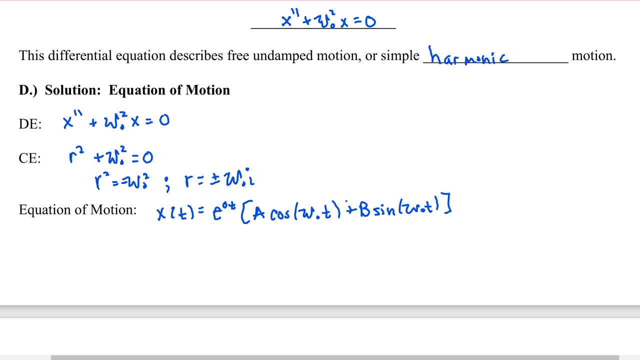 section how to express a general solution based on complex conjugate solutions. let's go ahead and simplify that. since e to the zero t is always one, we end up with a cosine of omega naught t- you're going to be tempted to put an x right there- and b sine of omega naught t. so the position: 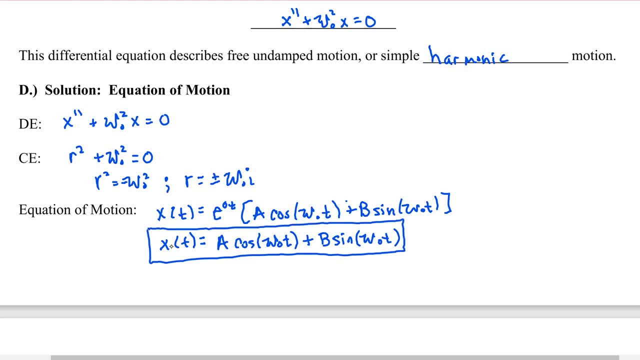 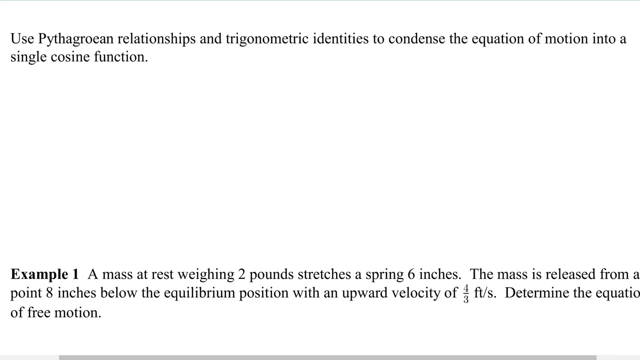 x of the mass above or below equilibrium position at any time t is now predictable by this equation of motion. this equation is very precise in determining the location of that mass at any time t. that's the beauty of mathematics: being able to precisely make predictions based on this analysis. now we're going to condense those two distinct terms into a single. 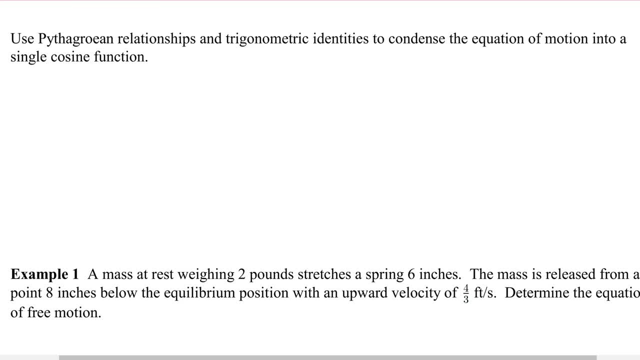 term using pythagorean relationships and trigonometric identities. so let's begin with a right triangle. suppose that my right triangle has an angle alpha and we're going to label the sides a, b and c. we can easily see from pythagorean theorem that c is equal to. 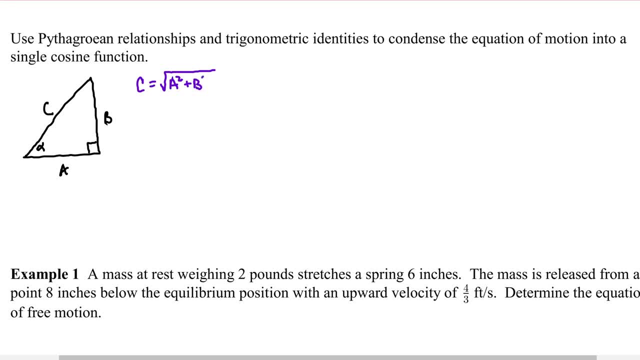 the square root of a squared plus b squared. Using SOHCAHTOA, we could make the observation that cosine of alpha think adjacent over hypotenuse, cosine of alpha would be a over c and sine of alpha so, or opposite, over hypotenuse would be b over c. Let's use these relationships. 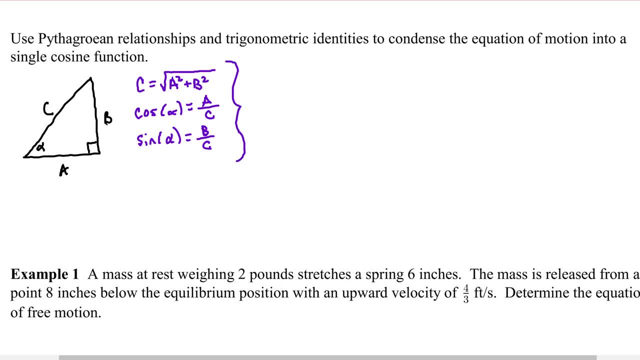 to condense our equation of free, undamped motion, Recall that x of t was equal to a cosine times omega naught t plus b sine times omega naught t. Based on our right triangle, we can observe that when we solve for a, a is c times cosine of alpha. so I'm going to replace this a with 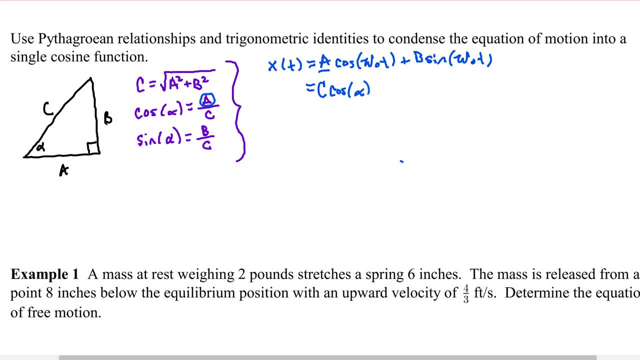 the expression c times cosine of alpha and I'm going to leave that second factor, cosine, omega, naught t. Second, here we have a, b. If we solve for b from our right triangle over here, b would be equal to c sine of alpha. so we'll replace b with c times sine of alpha and we'll leave the factor sine. 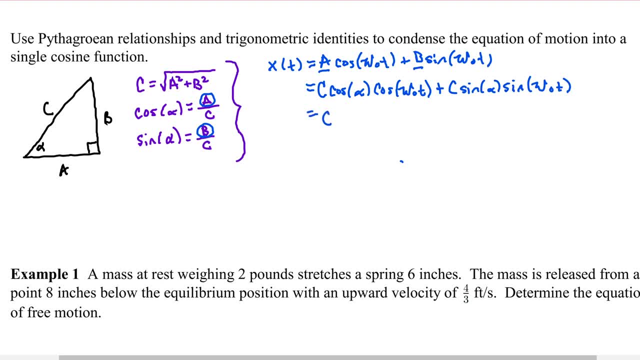 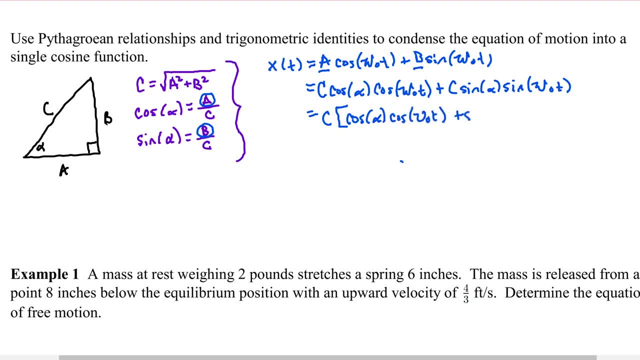 notice the pattern: cosine, cosine plus sine, sine. This can be replaced by c times cosine of alpha minus omega, naught t. That identity is simply called the cosine of a difference from trigonometry. Now recall also that cosine is an even function, So cosine of an angle is equal to cosine of the negative angle. 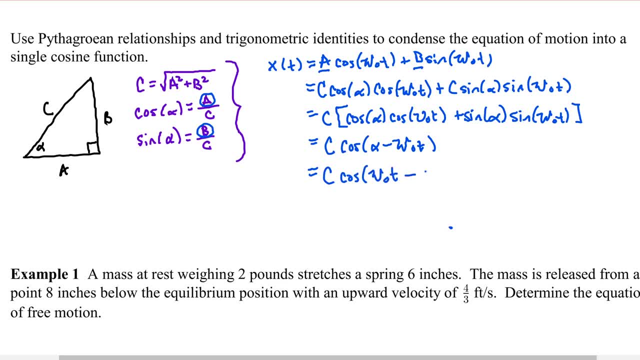 So I'm going to reverse these two terms around the difference. We know that is opposite by a sine, but it's going to yield the same cosine value. Then we can express our equation of motion as x of t equals c times cosine of. I'm going to factor out the omega naught here, leaving behind 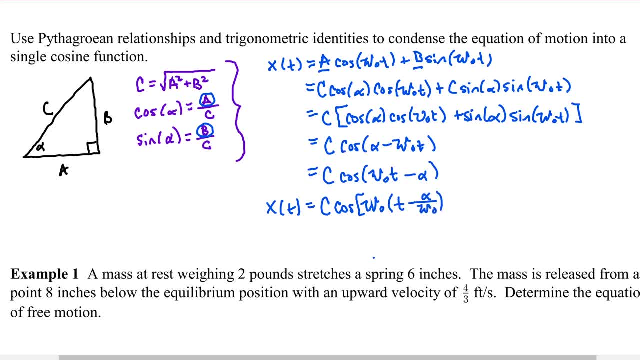 t minus alpha over omega naught. That's going to help me to identify transformations in the graph and begin to visualize not only the graph of this function but the motion of that harmonic oscillator. In this particular format, we can see that the amplitude of the mass is c. That's the 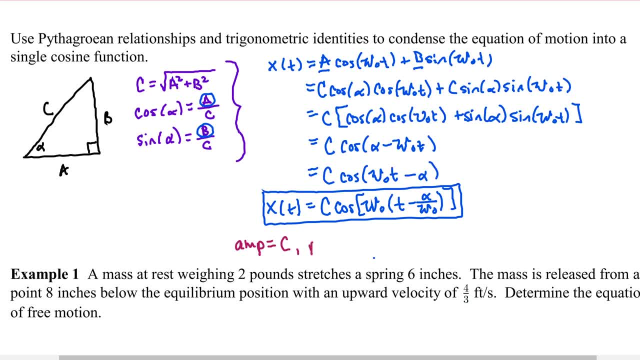 coefficient of our cosine function. The period of this function, usually denoted as capital T by this textbook, will be equal to the original period of cosine, which is always 2 pi divided by whatever coefficient lives right here. That's why we factored off that omega naught Just. 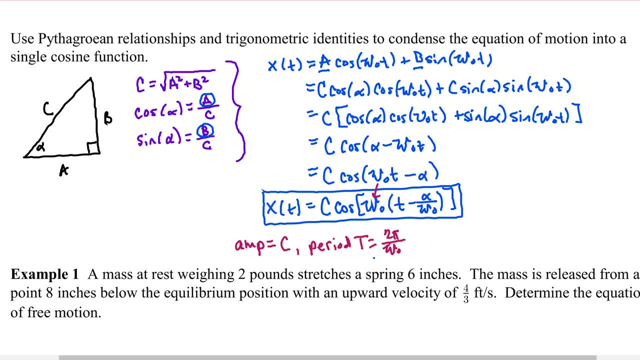 think about. how do you find the period of a cosine or a sine? Take 2 pi divided by the coefficient of the argument. So 2 pi divided by omega naught will give us the period of this wave. That's the length on the horizontal axis required for one fundamental cycle of. 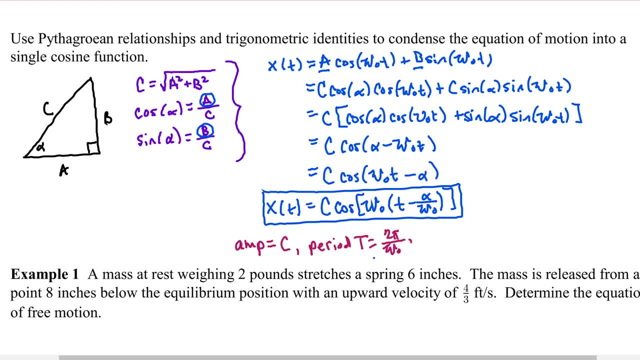 cosine to be completed. Now, strictly thinking about the graph, we can see that this cosine wave has a horizontal transformation of alpha over omega. naught, We're subtracting a number from the argument Again, that's just going to shift our cosine wave horizontally. Now. 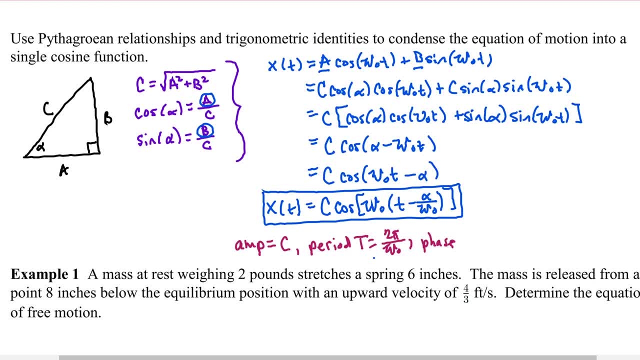 we're going to introduce some new vocabulary here. The phase angle is called alpha and that horizontal transformation that I mentioned, that's called the lag time. This is equal to alpha over omega naught. You'll want to be familiar with that terminology as you work. 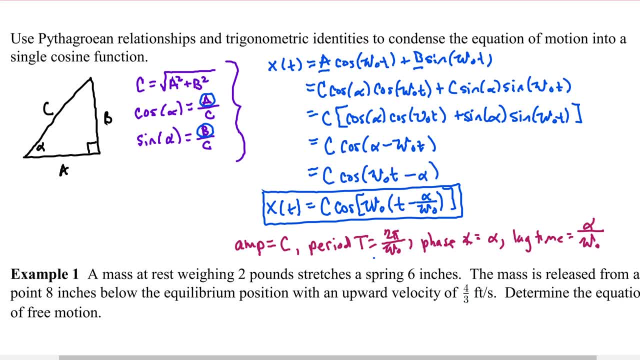 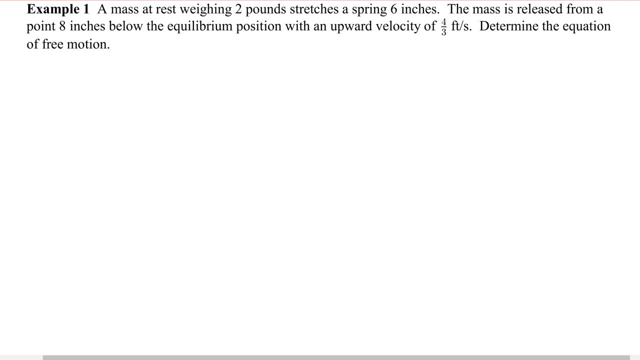 through your homework problems. So the lag time again, that's the horizontal transformation, That's the distance on the horizontal axis before one complete fundamental cycle of cosine begins. Let's go ahead and examine our first harmonic oscillator in example 1.. A mass at rest weighing. 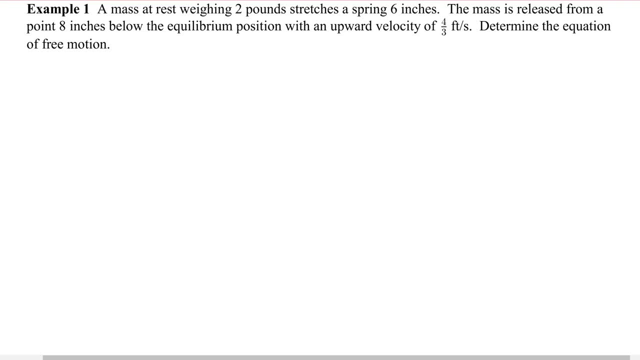 2 pounds stretches a circle of 2 pi over omega naught. This is equal to alpha over omega naught. The mass is released from a point 8 inches below the equilibrium position with an upward velocity of four-thirds of a foot per second. Determine the equation of free motion. So I'm 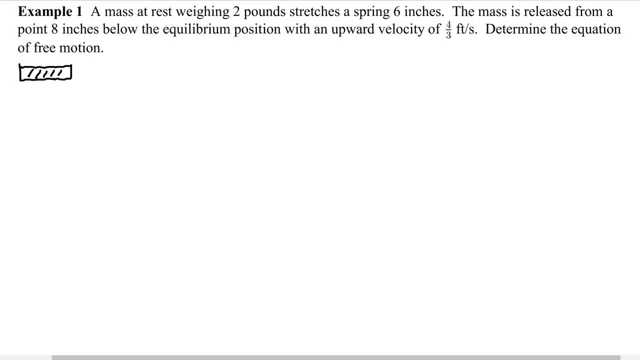 going to draw a picture again just to help us visualize the problem. So we start with a rigid base and we attach a spring to that base and our mass to that spring. Now we're told from the problem that the weight of the mass is equal to the spring. So we're going to draw a picture of a 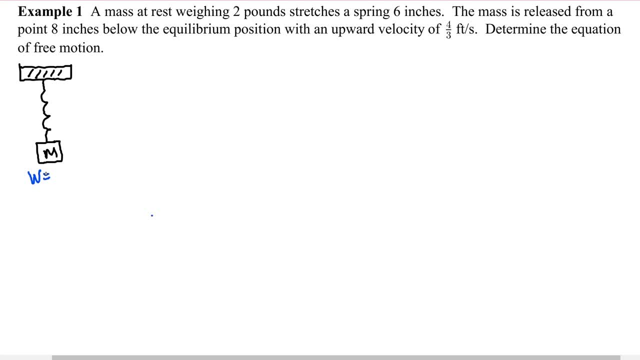 weight of this mass. not the mass, but the weight of this mass is two pounds and it's going to stretch the spring six inches. So whatever the length of the original spring was, our mass has stretched it an additional six inches and that is the equilibrium position, or static equilibrium. 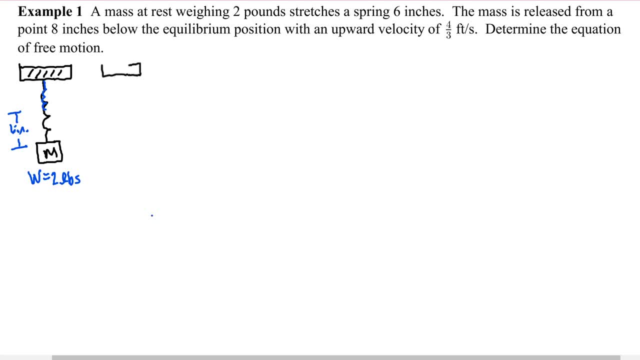 Then phase two: beyond static equilibrium. we're going to stretch the mass eight inches below equilibrium position. So if we visualize this horizontal line as static equilibrium, when we stretch the mass it's going to be eight inches below that initial resting spot, With that initial 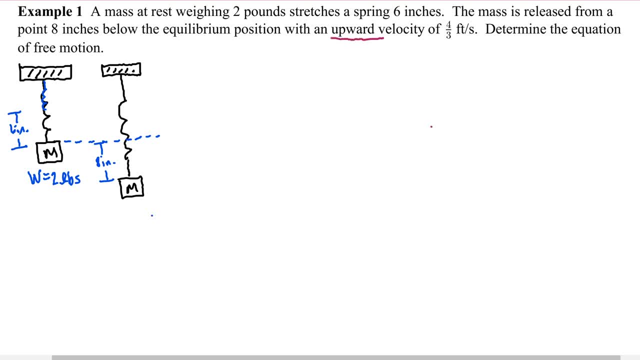 position. also notice that we're going to release the mass eight inches below that initial resting spot. We're going to release the mass with an upward velocity, so we're going to toss it up with an initial velocity of four-thirds of a foot per second. Our goal is to model this simple harmonic oscillator. 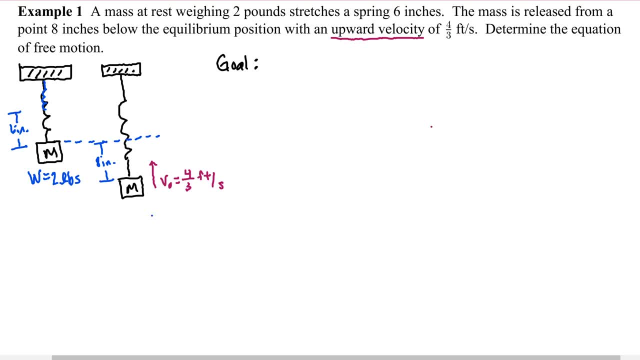 with a second-degree homogeneous linear differential equation with constant coefficients, That is, mx double prime plus kx equals zero. Now I'm reverting back to the original present of this model, as opposed to using the one with omega naught, It's usually simpler to set up like. 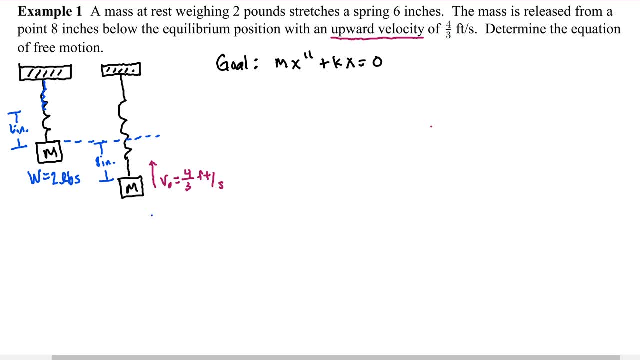 this and we use the omega naught simply to do the general analysis. So to write our model, we're going to need to find m and k. Let's start with finding mass. We need to find the mass. We are not told the mass, we are told the weight. Now recall: weight is equal to mass times weight. 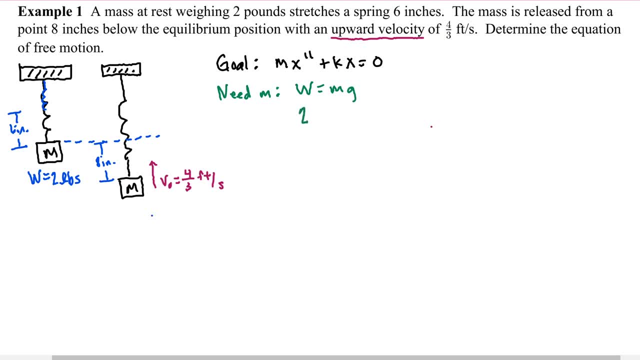 The weight here is 2 pounds, the mass is unknown and gravity is 32 feet per second squared, So it looks like our mass is 1: 16th. Now, just as a reminder about all of these units when you're. 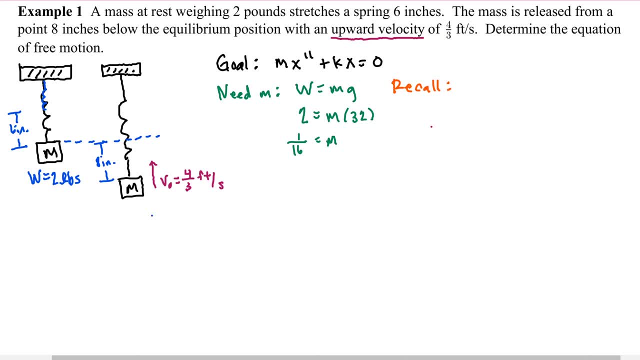 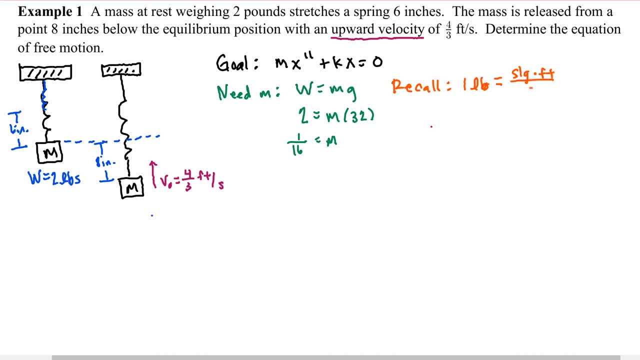 So 1 slug foot per second squared, okay, And similarly 1 slug- if I solve for it, would be 1 pound second squared per foot. So if I do a quick little dimensional analysis, we know that the weight is measured in pounds. gravity here is measured in feet per second squared. So when 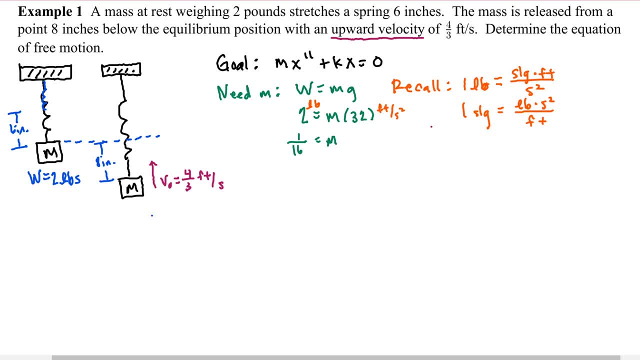 I divide both sides by 32 feet per second squared, I end up with units over here: pounds second squared per foot. okay, So the mass is 1 16th of a slug. Now that we've found m, let's work on finding k. 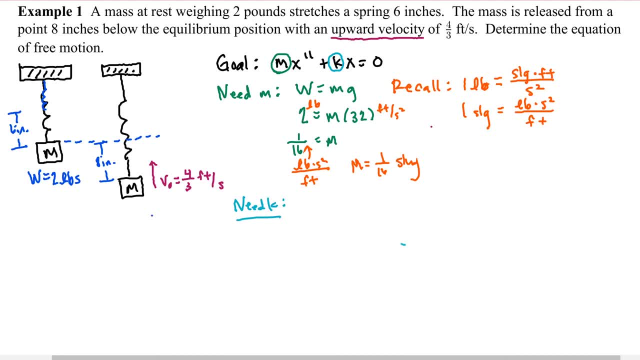 k is the spring constant. Recall from Hooke's law that the force in the spring is equal to negative k times x, Based on the weight of the mass. we know that the force in the spring is 2 pounds, but it's below equilibrium, So we'll say negative 2 equals negative, 2 pounds equals negative k. 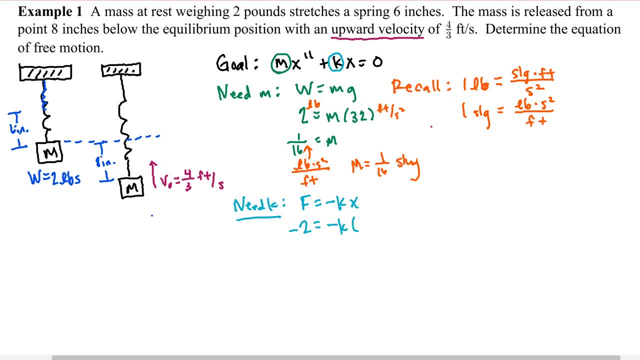 times x. x is going to be the position of the mass at static equilibrium. When the weight is 2 pounds, the length of our spring is 6 inches. Now, did you notice here that in our initial analysis we were looking at feet? 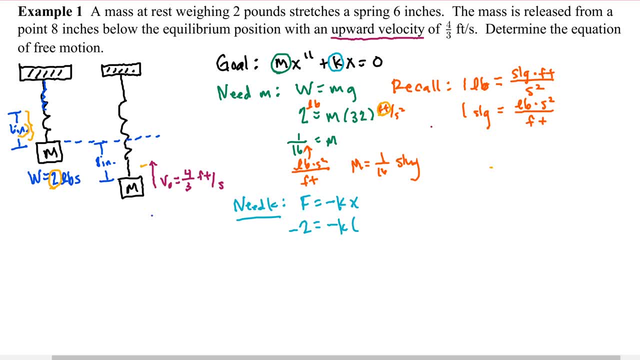 So we're going to add in feet. So here we have feet and we're going to add in our mass. So this is the second term and we're going to add in our mass, And so I'm going to take the last part of the unit and I'm going to put it all together. 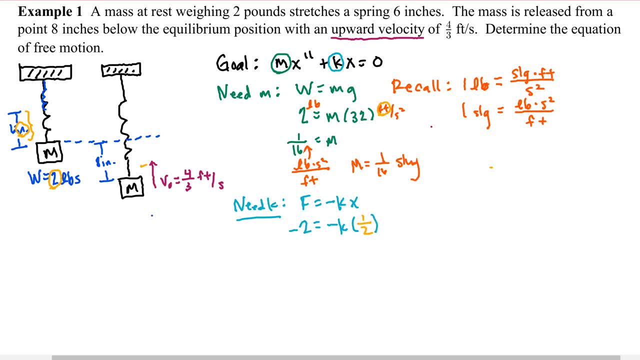 and we're going to get the average weight of the mass per second squared by 5 times x. This is the average weight of the mass. So by using this I got the average weight of the mass per second squared, just to have a good understanding. So 1 half is measured in feet, Remember. 2 was measured in. 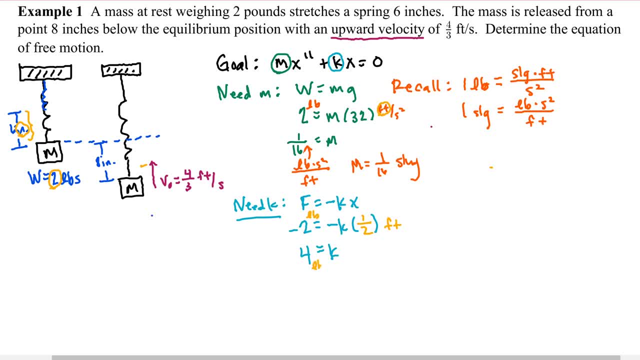 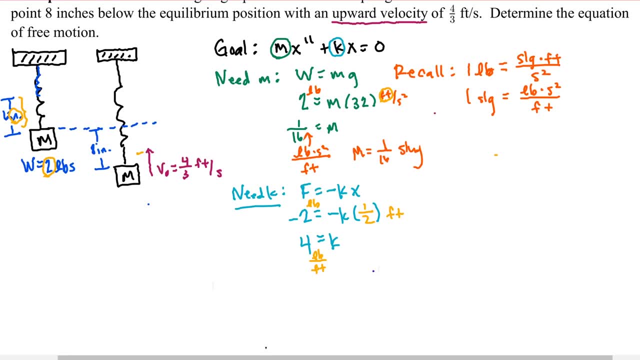 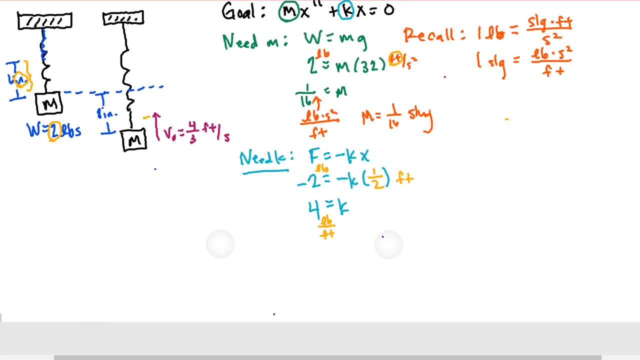 pounds. So the units associated with our spring constant would be pounds per foot. So k is equal to 4 pounds per foot. It's always a good idea to pay close attention to those units. You can work a problem over and over again. Can't figure out why you can't get it to work out. It might be the 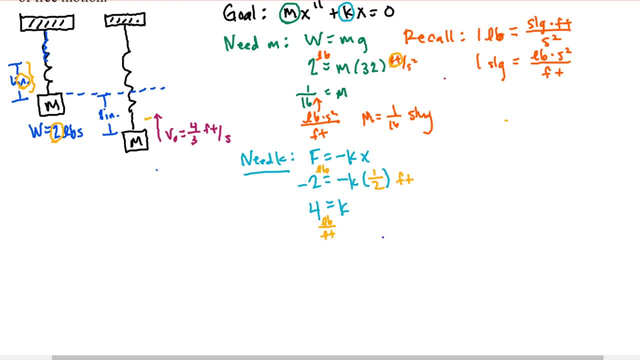 units. So please watch out for those dimensional differences. So we're ready to write our differential equation of motion. We're going to have mx double prime plus kx, equal to 0.. Remember, m is 1- 16th. So we have 1- 16th x double prime plus k, which is 4x equals 0.. Before we write our 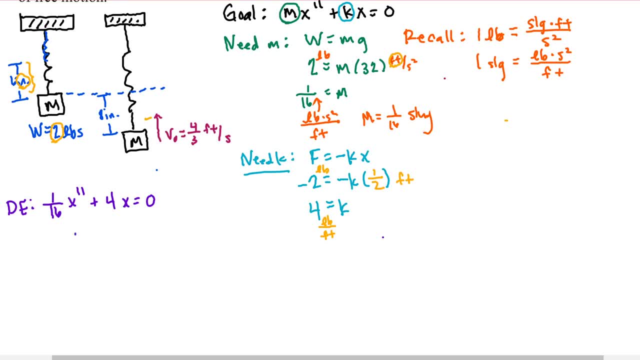 characteristic equation. let's make this really easy and multiply through by 16.. So we get x double prime plus kx equals 0.. So we have 1 16th x double prime plus kx equals 0.. So we have 1 16th x double. 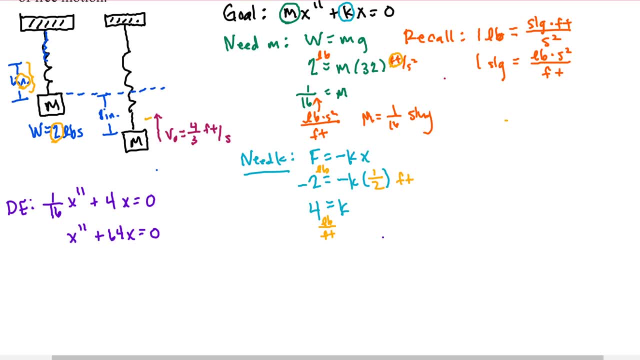 prime plus 64x equals 0.. Our characteristic equation is then: r squared plus 64 equals 0. And when we solve for r, we'll end up with plus or minus 8i. Thus our general solution would be: x of t equals e to the 0t times a cosine of 8t plus. 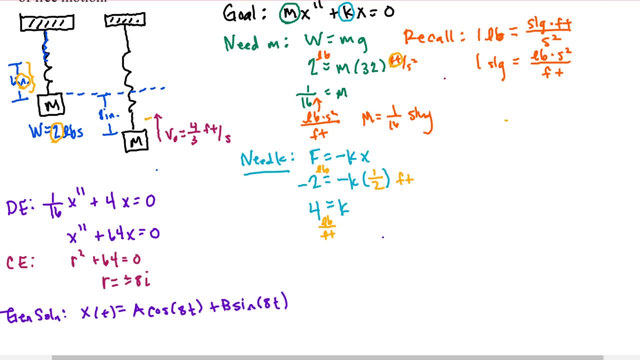 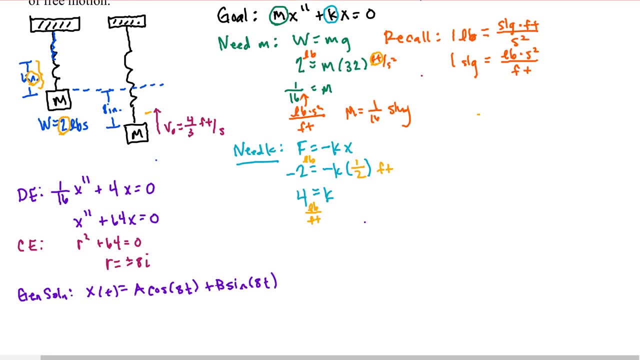 b sine of 8t. Remember that's how we handle the general solution when we have a complex conjugate pair of roots to the characteristic equation. At this point we need to proceed from our general solution to our particular solution. Recall that we have both initial position and. 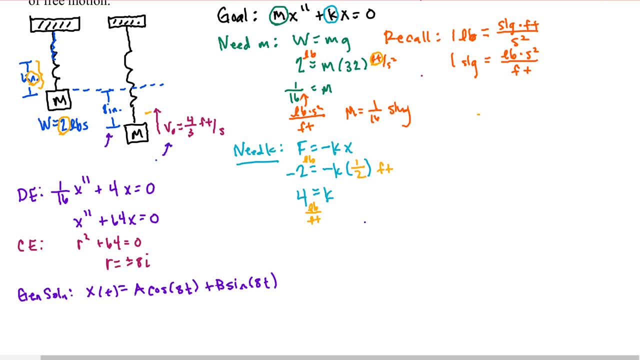 initial velocity. I've got two initial conditions that I can use to find my two unknown constants, a and b. One is initial position, one is initial velocity. So let's go ahead and take the opportunity to find our velocity function or x prime of t Differentiating. we're going to end up. 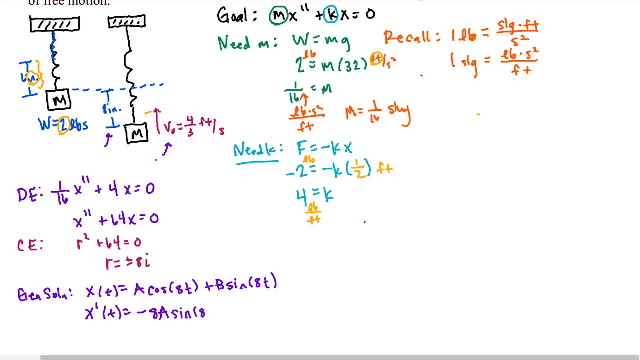 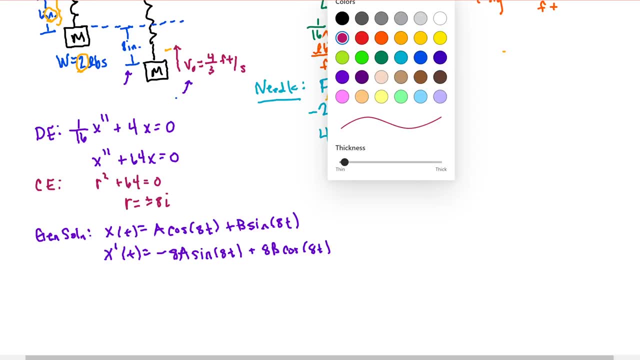 with negative 8a sine of 8t plus 8b cosine of 8t. Our initial conditions include initial position x of 0 equals. Now recall initial position x. naught was given in x prime of t. So we have x prime of t plus 8b sine of 8t. So we have x prime of t plus 8b cosine of 8t. 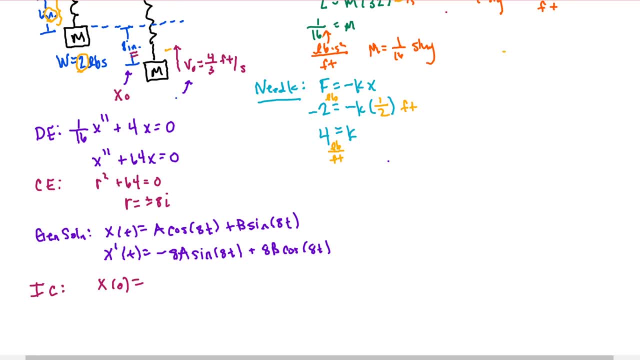 inches and we're going to need to convert that to feet. So if we think eight inches times one foot per 12 inches, we're going to get eight twelfths of a foot and when we reduce we end up with two thirds of a foot. for initial position X, prime of t or initial velocity that one was given in feet. 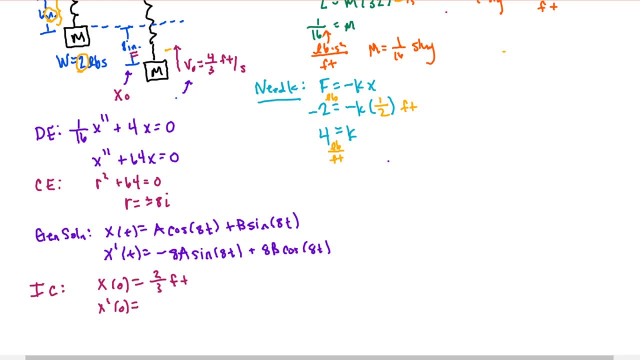 per second, The initial velocity. remember we toss the mass up a little bit, four thirds of a foot per second. Now, when the mass is in motion in an upwards direction, remember we're going to program that in as a compression of the spring or a negative value for position x, So upward velocity. 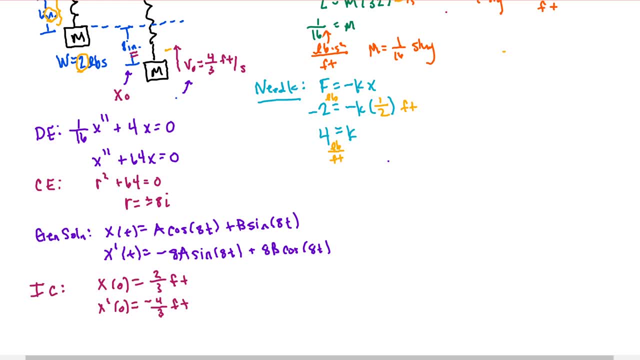 is paired with a negative sign. That's going to be a little more straightforward when we get to the horizontal model here in just a few minutes Now. with sine and cosine, these coefficients a and b are pretty easy to find. If we plug z zero in for t in these two positions we know that sine of zero is zero, so this whole term goes away. 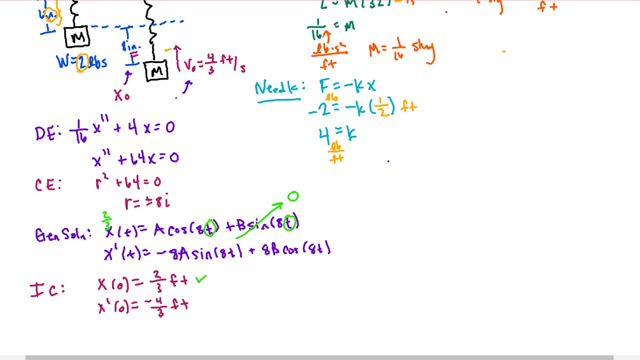 and if this is equal to two thirds of a foot, cosine of zero is one. so this would give us a equals two thirds. Similarly, we can plug zero in for t in our velocity function. Sine of zero is zero, cosine of zero is one. so if we set x prime of t equal to negative four thirds, 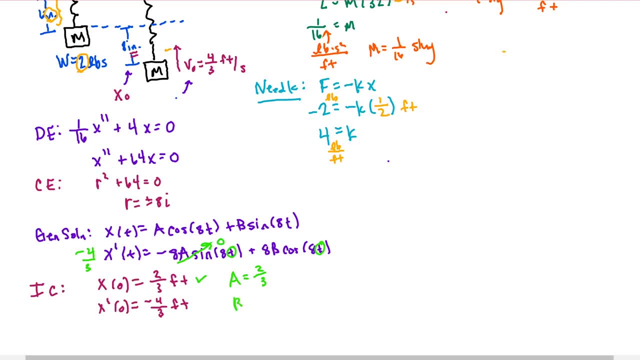 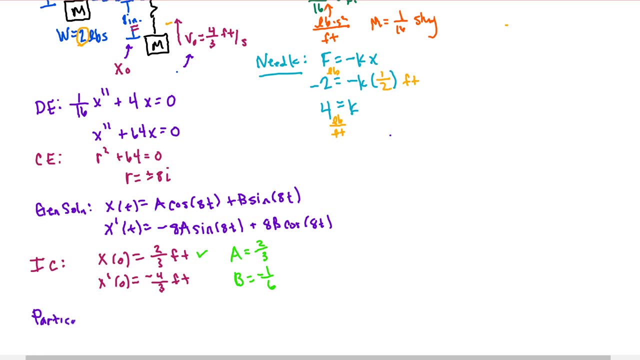 of a foot sine of zero plus t. we divide both sides by eight, We would find out b equals. This means that our particular solution is given by X of t, equal three thirds cosine of eight t minus one sixth sine of eight t. And this is the information that we would use here. We would do that out in a dry layer, in a densechied solution. 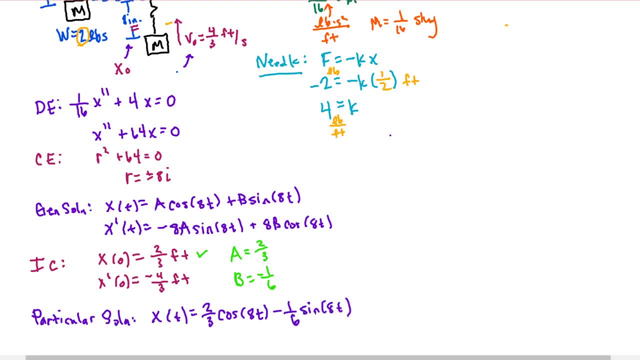 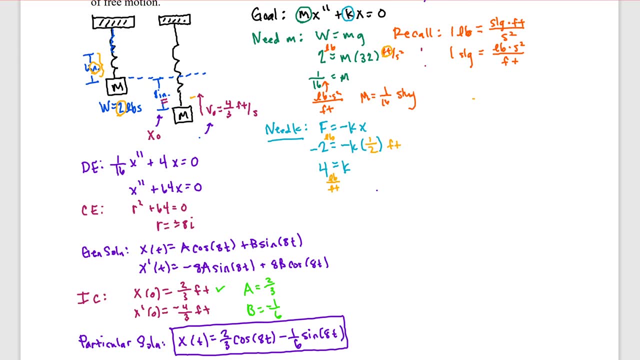 Again, we can plug zero in for t in this case. here We would find that b equals negative one. sixth ź is our equation of free undamped motion. this means, at any time, T. where T is measured in seconds, we can calculate the position of the mass either above or 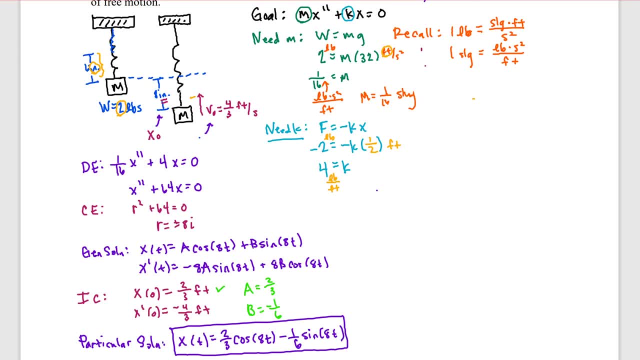 below that equilibrium position very specifically and accurately. remember: if the mass is in motion above the equilibrium position, we're going to get a negative position, negative velocity. when the mass is in motion below that equilibrium position, we're going to get a positive position or positive velocity. now let's go ahead and analyze this position function to really get an 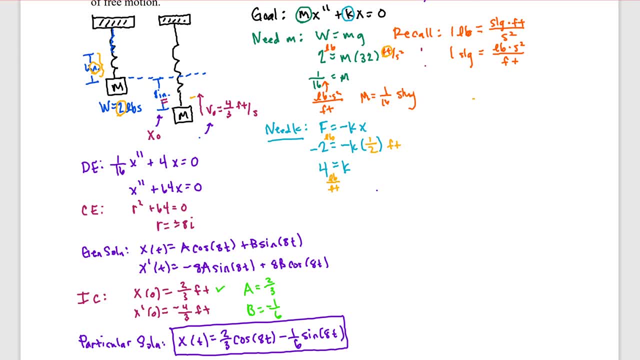 understanding of the behavior of this harmonic oscillator or this oscillating mass, let's see if we can calculate the amplitude of our mass. the amplitude, if you'll recall, is equal to the square root of a squared plus b squared. so the coefficient of cosine is a, the coefficient of sine. 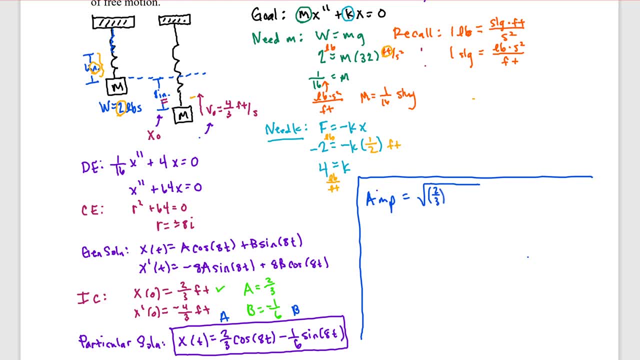 is B, so the amplitude will be the square root of 2, 3rd squared, plus negative 1, 6th squared, that's the square root of 4 9ths plus 1 over 36, or square root of 17 over 36, which gives me square root of 17 over 6, and this is in feet, so the 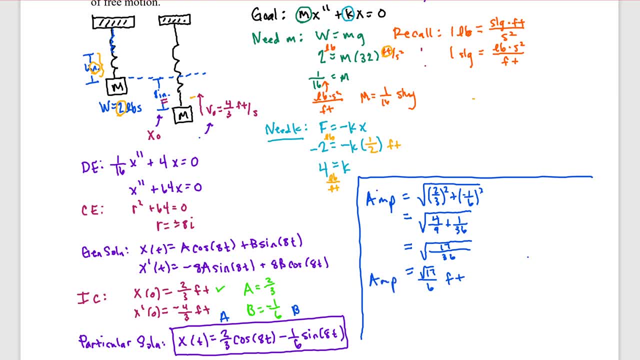 amplitude is square root of 17 over 6 feet and, by the way, this is approximately 0.068 feet. so that describes the maximum height of the mass above the equilibrium position and the maximum elongation, or the minimum point, the lowest point, of that mass below equilibrium position. let's figure out: 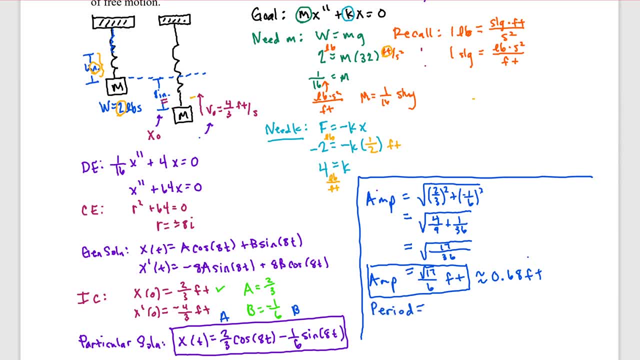 the period of this trig function. the period is 2 pi divided by the coefficient of the function of the trig function, and that is 3 pi divided by the coefficient of the function of the function of the function of the coefficient of the argument, or, in this case, pi over 4.. This is a unitless measurement or you can. 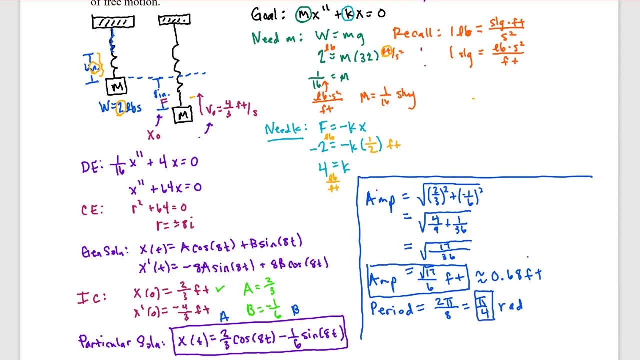 think of that in radians. So the distance pi over 4 on the horizontal axis is required for one fundamental cycle of cosine to occur. If we invert this number, by the way, we're going to get the frequency or the number of cycles per one unit. So 4 divided by pi gives us approximately 1.27. 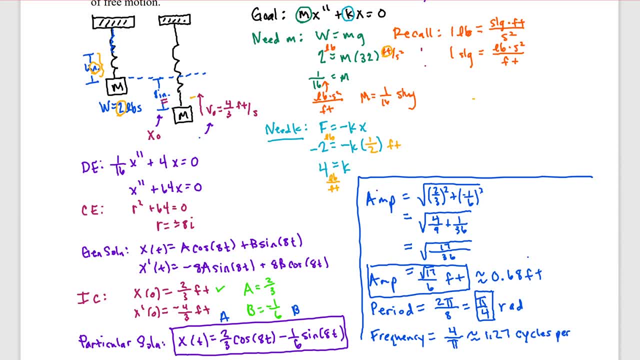 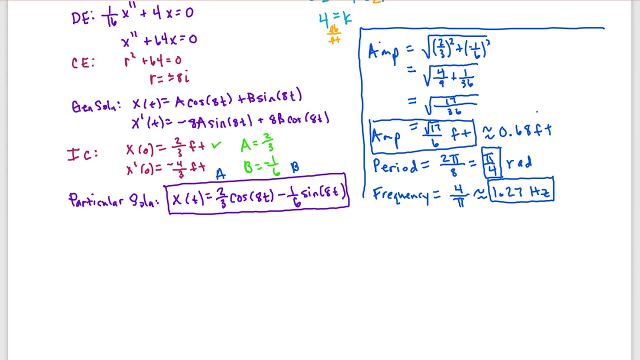 cycles per second. And, by the way, cycles per second is another way of saying hertz. So 1.27 hertz would be the frequency of this oscillating mass. This means that the mass is going to complete the cycle, So we're going to get the frequency of this oscillating mass. 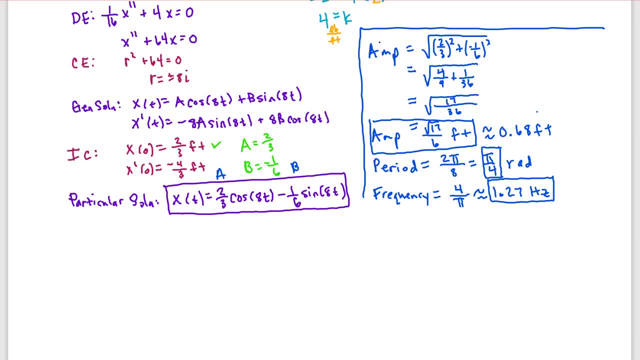 a little over one complete oscillation in one second. Now, if you'll recall from our analysis, when we set up our right triangle with angle alpha here- horizontal segment A, vertical segment B and hypotenuse C- we said that alpha was equal to the phase angle To figure out this value. 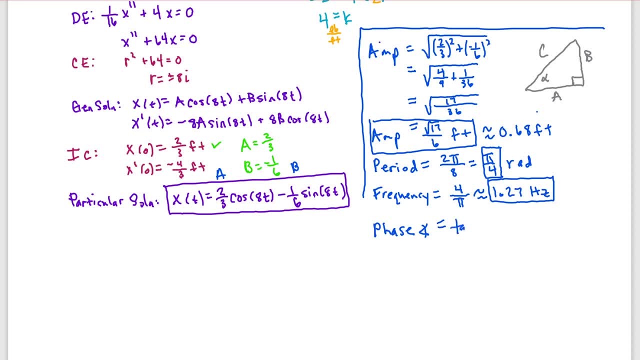 we can simply use our right triangle. Notice: inverse tangent of B over A will give us alpha. B in this problem is negative one-sixth, A is two-thirds. So with our calculator in radian mode we would obtain the value negative 0.24 radians. Or, if we want to see that in a. 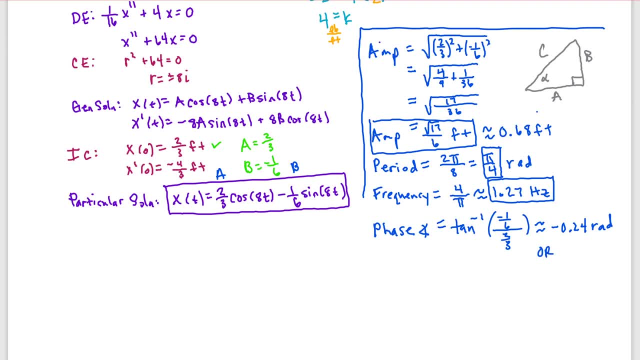 positive value. we could add 2 pi to that and that would give us 6.04 radians. If we want to look at the positive side of the x-axis, we could add 2 pi to that and that would give us 6.04 radians. 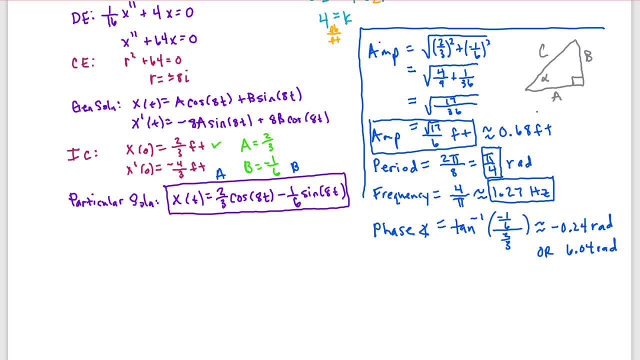 Or the horizontal axis. that gives me a positive time. And finally we can find the lag time. Remember, this is equivalent to the horizontal shift of that cosine wave. We defined it as alpha over omega naught. Alpha here is approximately 6.04 radians Omega naught. 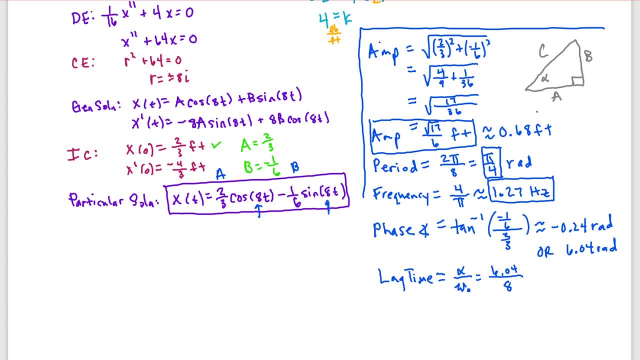 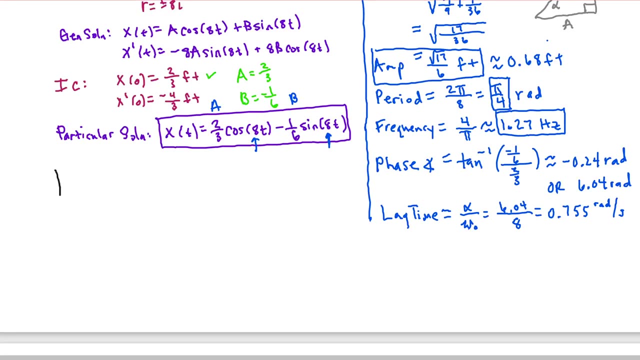 by the way, lives right here. It's the coefficient of the argument, So we could approximate this to 0.755 radians per second. Now let's go ahead and construct a pretty detailed graph of this position function, with all that information on display, So we'll have a good understanding of 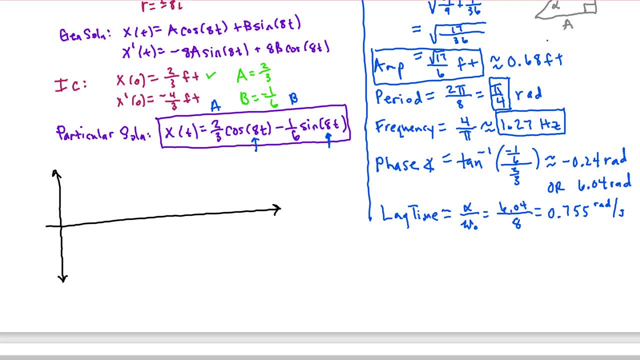 what all of those individual things mean. On the horizontal axis, we're going to have time in seconds. On the vertical axis, we'll have position in feet. Recall that a positive position function is a positive position function, So we're going to have a positive position. 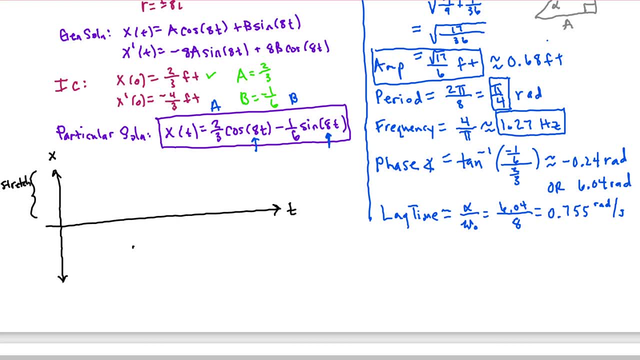 indicates that the spring has been stretched And this is motion in the downward direction. And if x is negative, the spring is in compression And this indicates the mass has moved up. So it's a little bit counterintuitive. I'm going to measure up to 1 and down to negative 1 and recognize that. 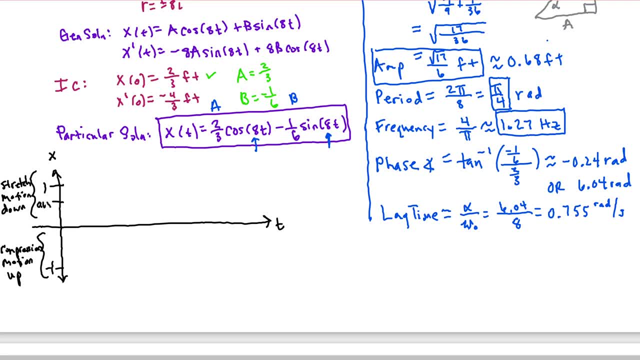 the amplitude of this function is 0.68.. So the highest it's going to go is 0.68 and the lowest is negative 0.68.. Now the period is pi over 4.. So we know that it's going to take a distance of pi over. 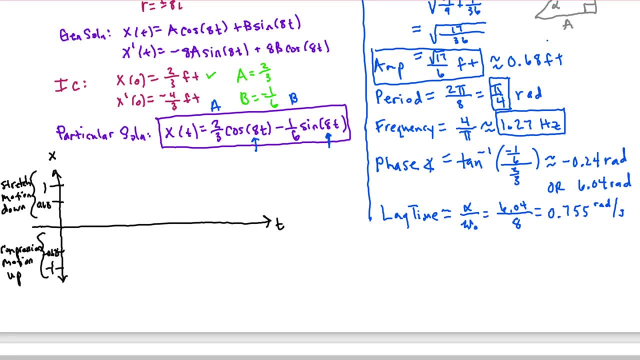 4 for our cosine wave to make one fundamental cycle. And if you'll recall, from trig generally, you graph five key points where you have four subdivisions of your period to make a very clear integral. So I'm going to label my t-axis in multiples of pi over 16.. So that is 1 fourth of. 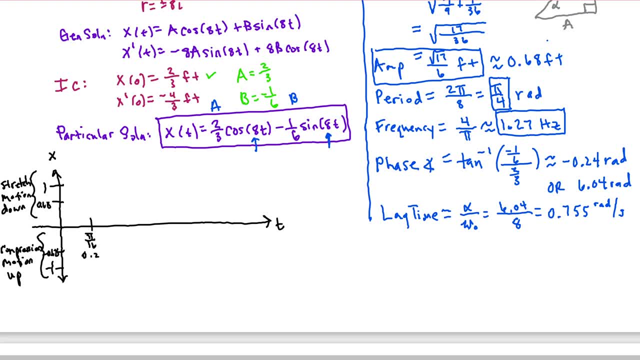 pi over 4.. Pi over 16 is about 0.2.. I'm going to approximate these so we can compare with our approximations. Next one would be pi over 8.. Pi over 8 is approximately 0.4.. Then we'd have 3 pi. 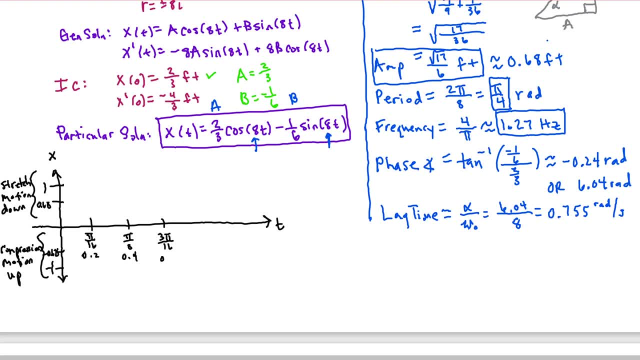 over 16.. That's approximately 0.6.. And then, finally, our pi over 4, which is approximately 0.8.. Notice our lag time, which represents our horizontal shift, is approximately 0.8.. It's just to the left of it. So our phase shift here, I'm sorry. 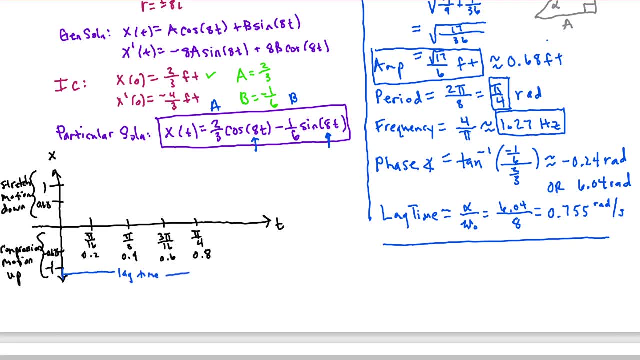 our lag time indicates a drag before we get one complete fundamental cycle of our cosine wave. So our cosine wave is going to begin right here. So, just approximating our points, we can sketch in a cosine wave, remembering that our initial position was just below the maximum. 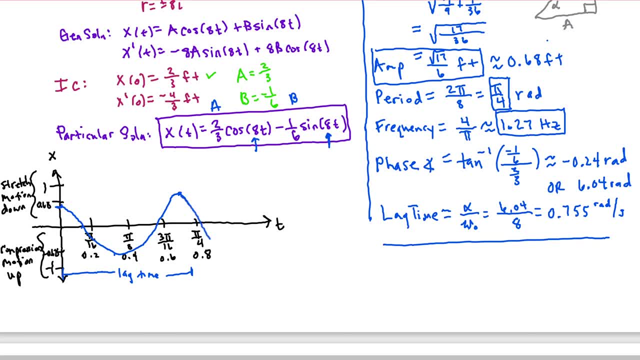 amplitude there. So if we were to continue this then we would see that complete cosine fundamental cycle. What we see during the phase called the lag time is part of a fundamental cycle of cosine. The maximum is going to be over here somewhere, So I can see that bowl shape right. 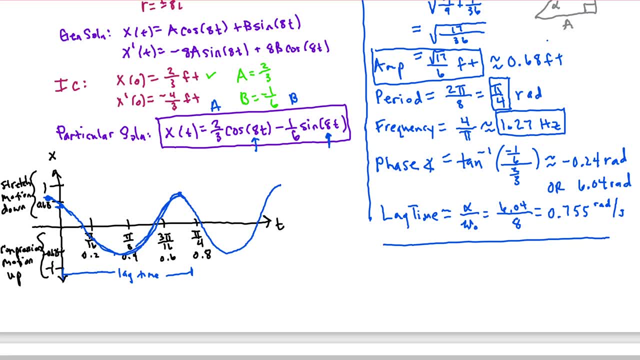 here Again, it's shifted just a little bit. You'll very likely want to examine this with your calculator. Let me remind you, put your calculator in radian mode so that it'll match up with the units that we have here Now. the domain of this function is negative infinity to infinity Of. 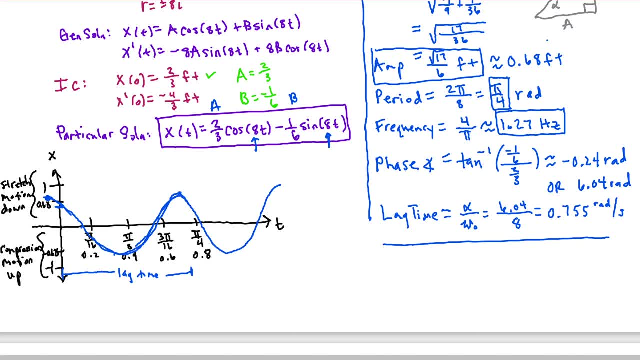 course, what's relative to our experiment would be: the interval from t equals 0 to infinity, so positive time only. But observe that this cosine wave continues oscillating forever and ever and ever, without ever stopping. So this means that our mass is oscillating up and down forever and ever without ever slowing down. coming back to 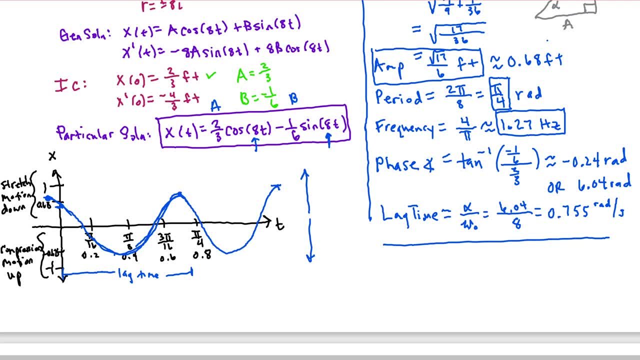 equilibrium position and stopping. There's no external or damping forces working on this simple harmonic oscillator, So this is again free, undamped motion. And next we're going to consider adding a little bit of reality into this experiment. So we're going to start with the 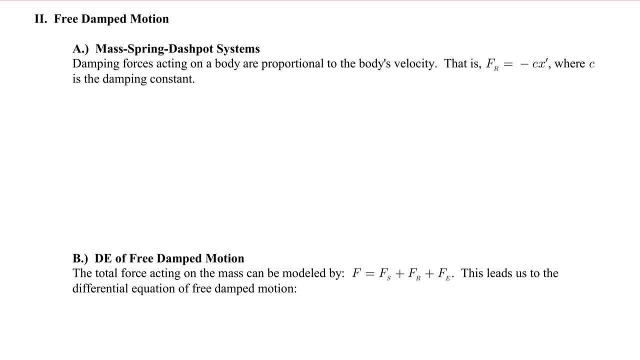 moment We're going to make a couple of important changes for part two of our notes. Next we're going to study free damped motion. So it's still free motion. That means there's no external interference with the rigid base for our spring. But this is damped motion, so there will be. 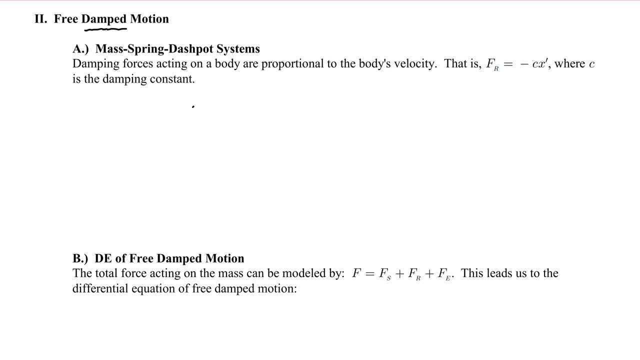 resistance to the velocity of our mass. The second change that we're going to make is we're going to examine a horizontal model in this case. So part A, we're looking at a mass spring dashpot system. Damping forces acting on a body are proportional to the body's velocity. 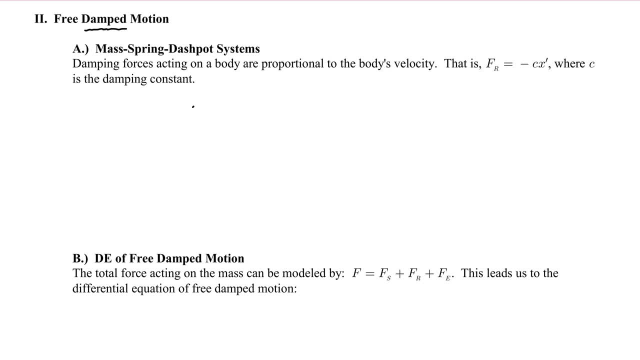 That is f sub r. so the retarding forces are equal to negative c x prime. x prime is the velocity of the oscillating mass and c is what we call a damping constant. These retarding forces are in the opposite direction of the body's velocity, so they're resisting forces For a. 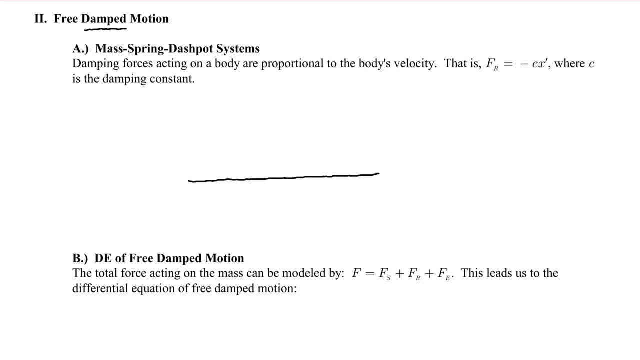 horizontal model. we'll examine a horizontal model. We'll examine a horizontal model and we'll examine a surface which will be nearly frictionless, essentially frictionless for our experiment. We'll have a rigid support on the left side and a rigid support on the right side. 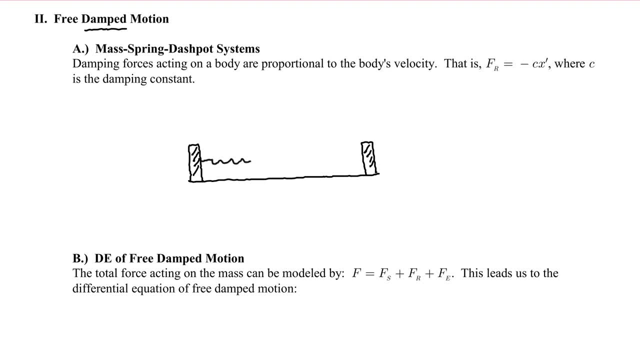 We'll attach a spring to this support. but here we're going to have a mass oscillating on this essentially frictionless surface. Now, if I compress the mass this way, the spring has the same effect as it did in the vertical case: It's going to want to exert a 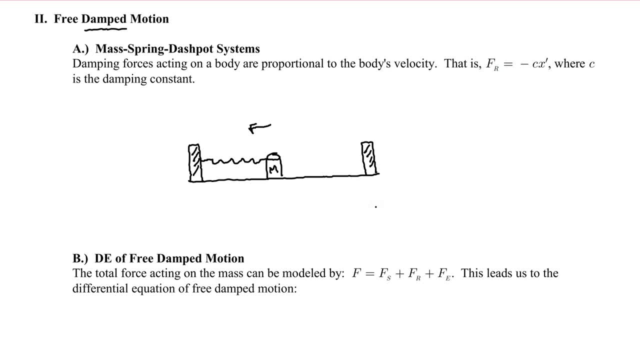 restoring force on that mass and move it back into equilibrium position. If I pull the mass this direction, the spring is going to want to pull it right back into that equilibrium position. But what we're going to do in this case is attach on this side something called a dashpot. You can 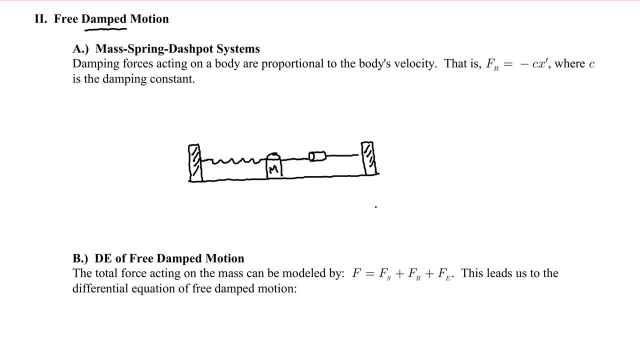 think of that like a little shock absorber. So it's going to resist the velocity of this mass. this little object is the dashpot, or you can think of it as shock absorber. My kids used to have a zipline in the backyard from a tree to a pole and there was a little. 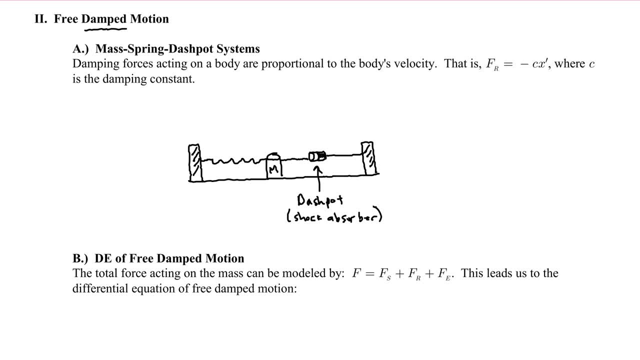 break on that zipline, which reminded me of this experiment. It was a dashpot. It resisted the velocity of my kiddos hitting the other pole. It really worked like a charm. Now our equilibrium position is going to be a little bit different, So we're going to have a little break on that zipline. 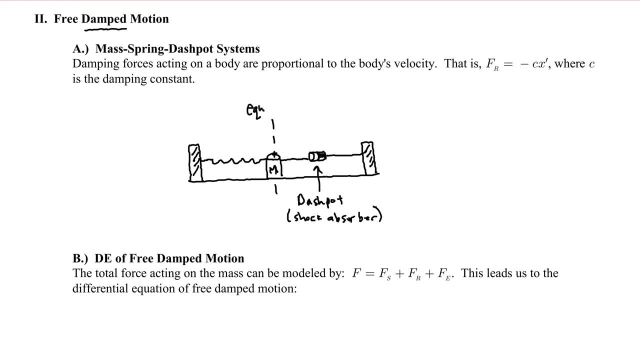 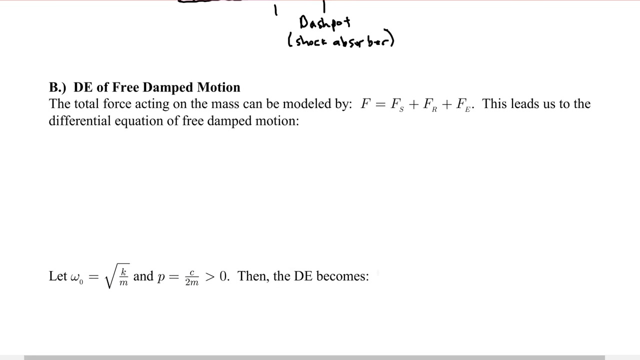 ats. The other thing I like about this particular model is that motion to the right will be modeled by a positive position, since that will elongate the spring, And motion to the left will be a negative position, since that will compress the spring model. Newton's second law regarding acceleration, as well as Hooke's law, still comes into play here. 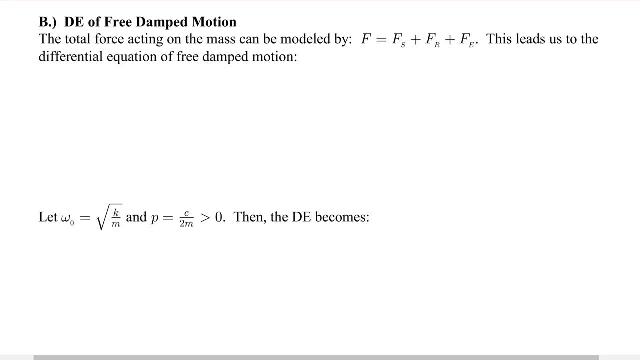 but now we're going to program in the resistance to that velocity. So let's write the differential equation of free damped motion. The total force acting on the mass can be modeled by F. F is the total force equal to the force of the spring, plus the retarding force or the resisting force. 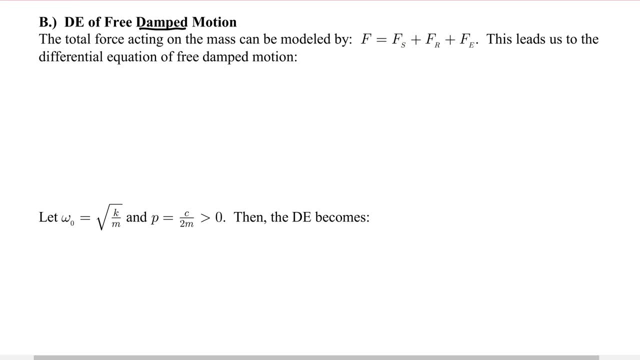 plus any external forces. This leads us to the differential equation of free damped motion. The total forces acting on the spring can be equated to mass times, acceleration, mx, double prime. This is equal to the force in the spring that comes from Hooke's law, negative kx plus the 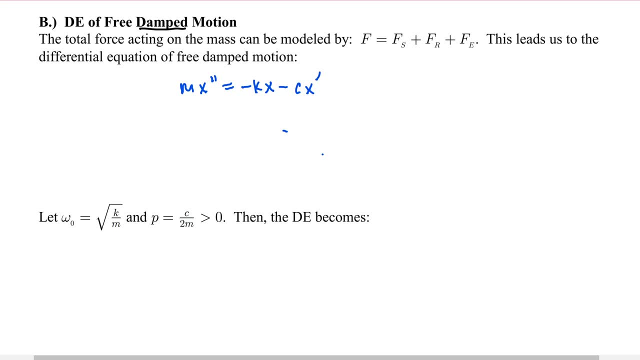 retarding force, that's the damping constant times velocity, plus any external forces acting on the spring. We'll call that F of t. for now, Rearranging our equation gives us mx double prime plus kx. actually, let's go cx prime next, plus kx equals F of t With the presence of this, 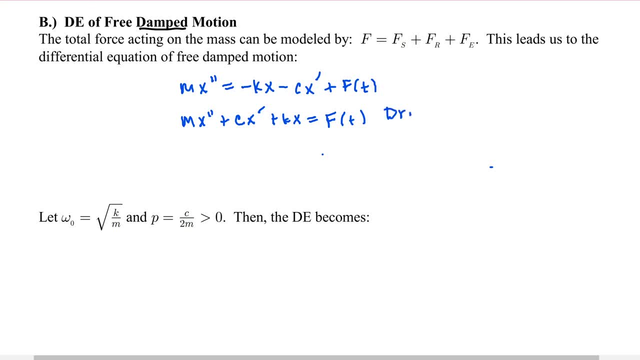 function of t on the right side. this is called driven motion, and if that is the case, then we're going to have a function of t on the right side which is zero over there on the right side, which it will be for our experiment. This is called free. 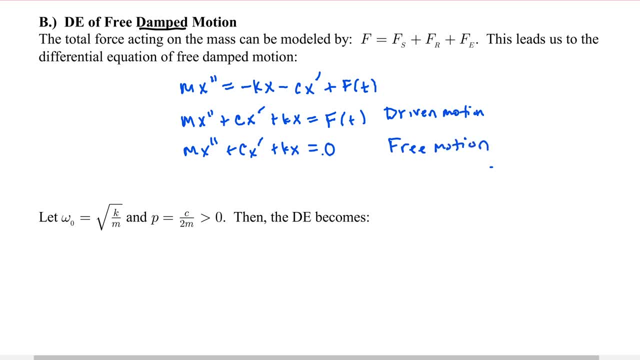 motion. So eventually we'll have that right side added in. For now we are examining free motion. Free motion simply means there's no external forces acting on the rigid bases or the rigid supports for our setup. but we do have resistance to the velocity. So this is free damped. 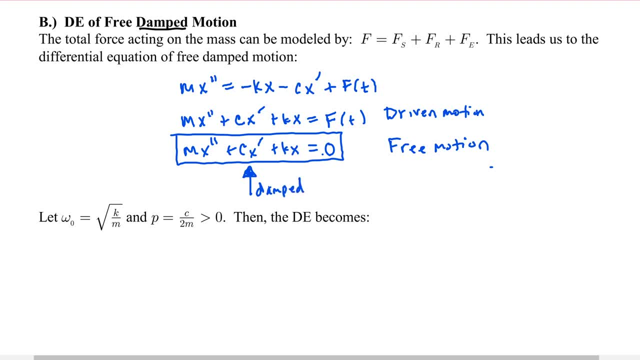 motion, So it's going to cause that oscillation to slow down a little bit. Our next goal is to go ahead and solve this differential equation in general. So, as we did before, we'll let omega naught equal the square root of k over m and we're going to define another constant. 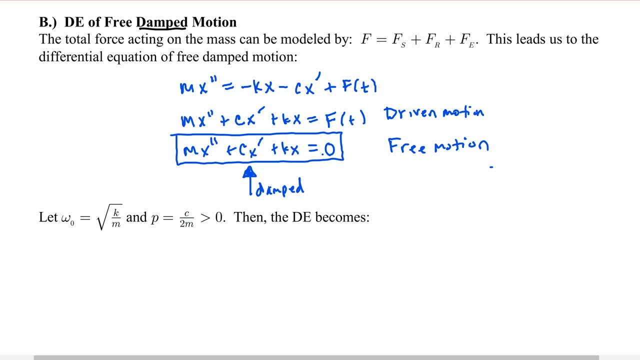 p equal to c over 2m, which is a positive constant. Again, that will be for convenience of our general solution. Then the differential equation which originally is mx double prime plus cx prime plus kx equals zero. If we divide through by m, we get x double prime. 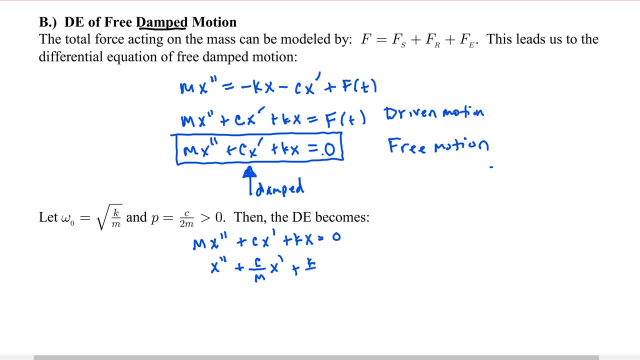 plus c over mx prime, plus k over mx, equals zero. Then we can see with our defined constants: c over 2m is equal to p. so c over m must be 2p, And k over m once again becomes omega naught squared times 2p. 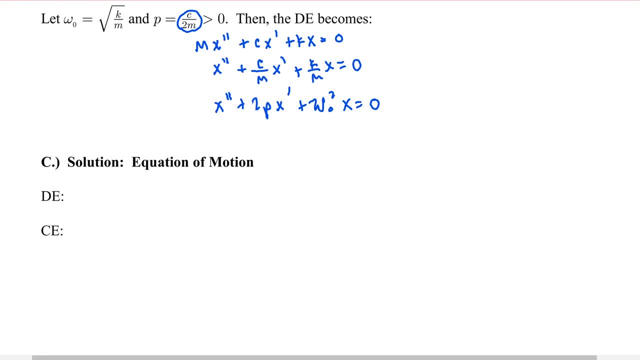 Let's go ahead and find the solution to this equation of motion. The differential equation that we'll solve in general is x double prime plus 2px prime plus omega. naught squared, x equals zero. By the way, when we construct our models, we'll generally follow this format. 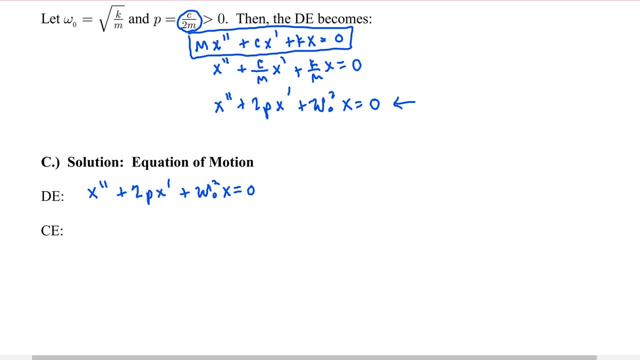 but again, we're using this format for our analysis. The corresponding characteristic equation is therefore r squared plus 2pr plus omega, naught squared equals zero. We need to find the roots of this characteristic equation. So we're going to get two solutions- r sub 1 and r sub 2, and we can simply apply. 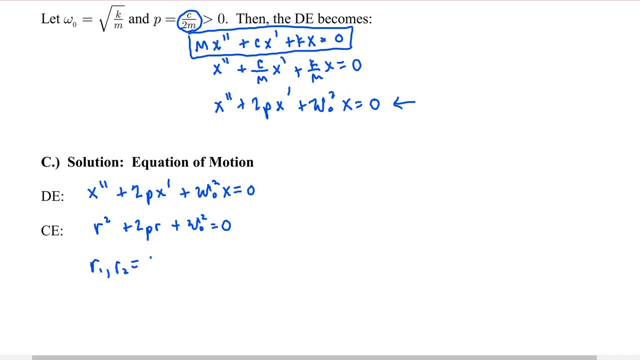 the quadratic formula to find these roots. So we'll have negative b, that's negative 2p, plus or minus the square root of b squared, that's 2p squared minus 4 times a, which is 1.. C, which is omega naught, squared all divided by 2 times a or 2 times 1.. We need to determine. 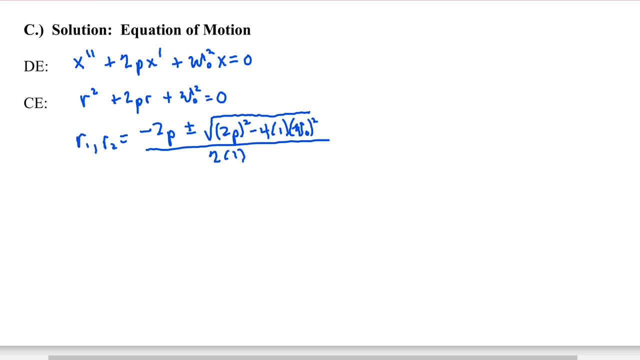 if we're dealing with distinct real solutions or if we're looking at a complex conjugate pair. So let's go ahead and simplify. Working underneath our radical, we're going to find out. we have 4p squared minus 4 omega naught squared, all divided by 2.. Let's go ahead. 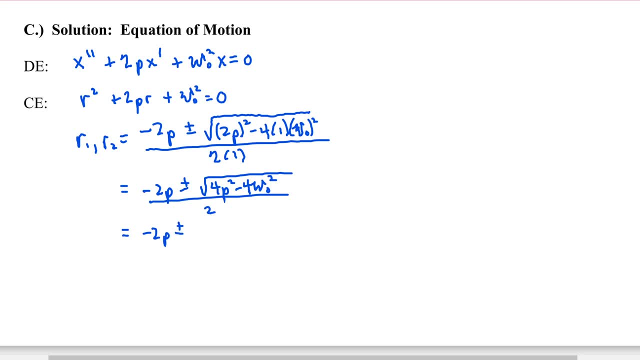 and factor out the 4 from the two terms underneath. Remember the radical, and we know the square root of 4 is 2, so we end up with p squared minus omega naught squared. Both of the terms in the numerator are divisible by 2, so we 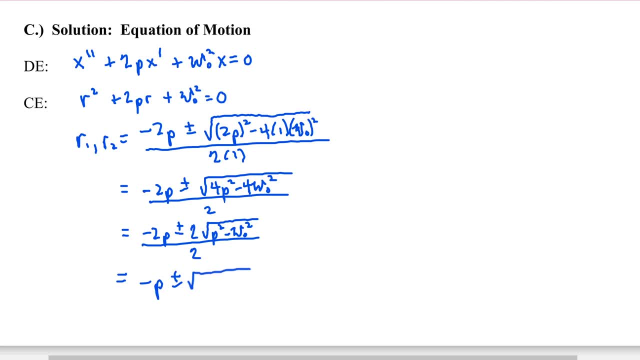 end up with negative p plus or minus. the square root of p squared minus omega naught squared. Once again, the nature of these roots will indicate how we should express the general solution. So we need to know: are they real distinct roots or are we dealing? 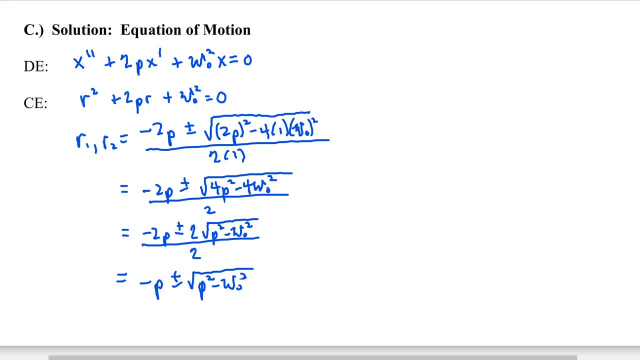 with a repeated real root or a complex conjugate pair. In order to make that call in this general case, we need to know the sign of the discriminant. Remember, the discriminant is the number under that radical or the radicand. This is going to lead us to three different cases based. 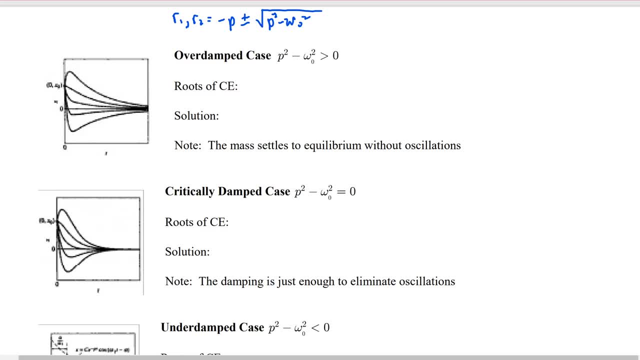 on the sign of that discriminant. Let's examine the first case. Suppose that that discriminant, p squared minus omega naught squared, is greater than 0. That is, it is positive. If it's positive, then the square root of that number would be a real number. 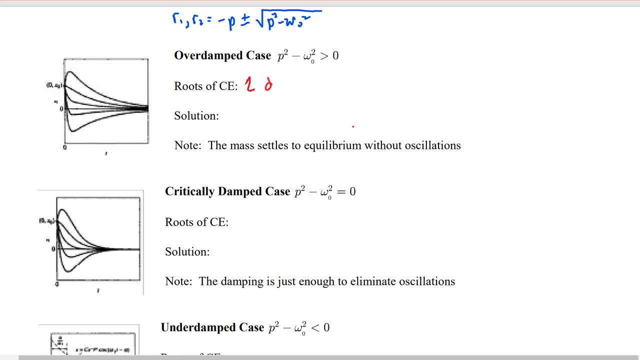 So we would end up with two distinct real solutions. This means that we would express the general solution as: x of t equals c sub 1 e to the whatever r sub 1 comes out to be. so we would simplify those numbers plus c sub 2 e to the r sub 2 t. 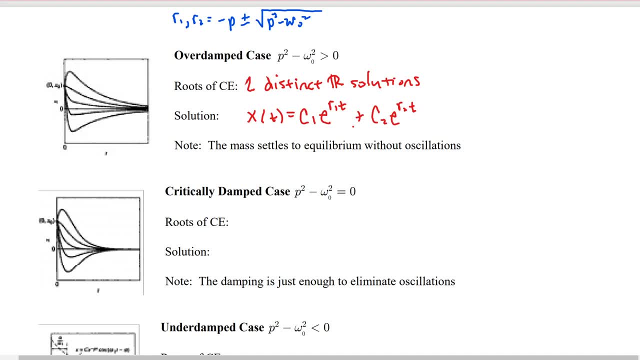 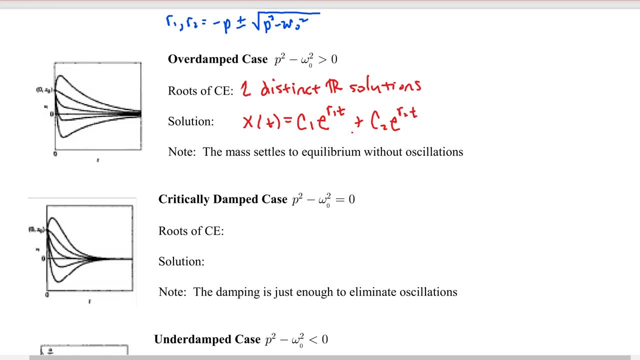 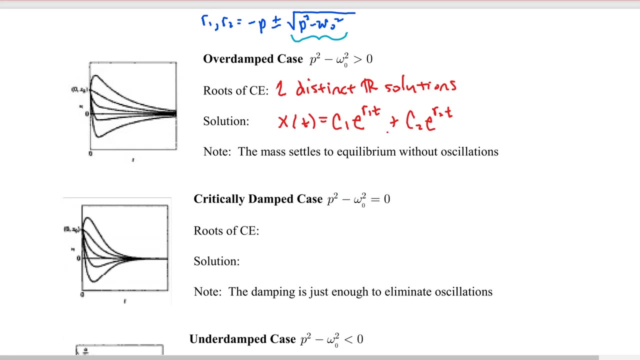 Now an important thing to observe about both r sub 1 and r sub 2,: if p squared minus omega naught squared is in fact positive, then this number right here is going to be smaller than p, If I think about taking p and squared. 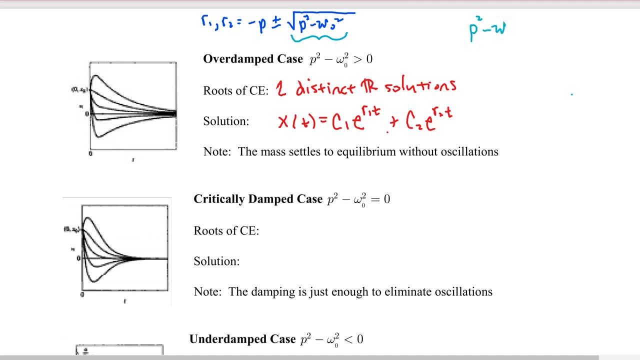 and then subtracting a number from it, that's going to cause the value under the radical to be smaller than p. For example, if omega naught squared were to be 0, the square root of p squared is just p. So since I'm subtracting a number from p squared and then taking the square root of it, 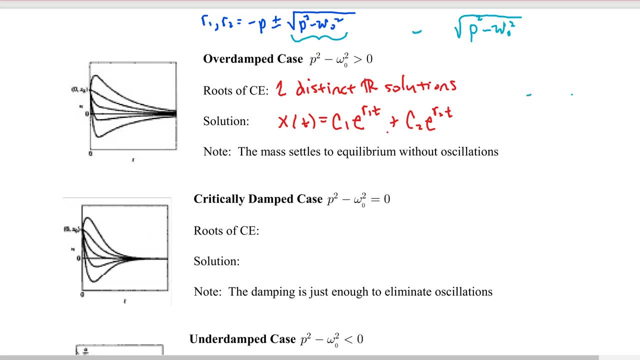 we can see that that radical is smaller than p. So if I take a number- negative p- and I add a number smaller- smaller than itself, I'm going to get a negative number. So my first root is a negative number. Now, if I take a negative number and then subtract more from it, 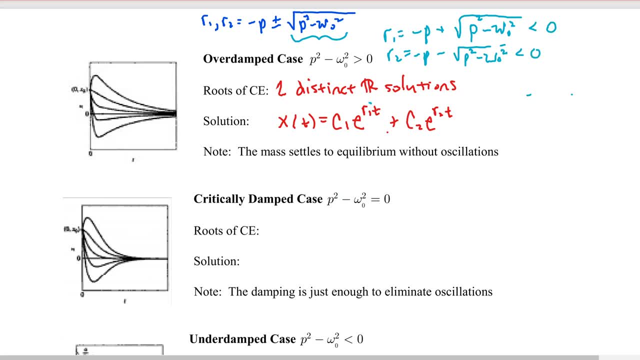 I still have a negative number. So both of these exponents are negative. That means they are exponentially decreasing. This is what we call the overdamped case, That is, the resistance to the velocity is so strong that the mass is simply going to settle to its equilibrium without oscillations. 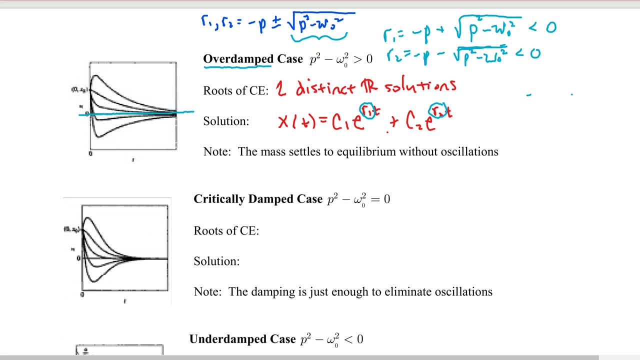 If I remember the equilibrium position to be modeled here by the horizontal axis, even if I take that mass and I toss it to the right with a positive velocity because of the damping it's going to immediately settle back down to equilibrium position. It's not going to cross through equilibrium and oscillate. 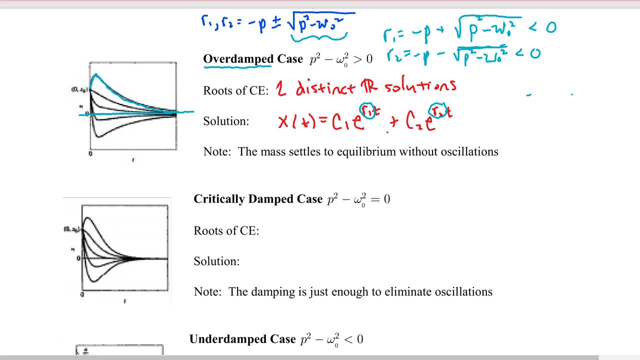 It's just going to settle very slowly back down to its equilibrium position. So if I take a negative number, negative p squared, and I add a number smaller than p squared, it's going to move very slowly back down to equilibrium position. Or if I consider a different set of initial conditions, 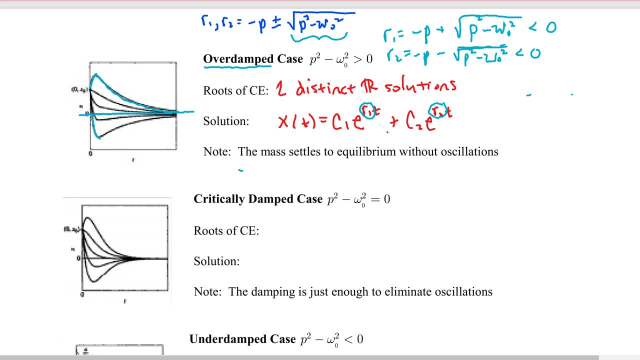 let's suppose I toss that mass to the left with a strong velocity. Well, because of the shock absorber, because of the damping there, the mass is going to turn around and settle down back to its equilibrium position. It's going to be moving very slowly because the resistance is overdamped. 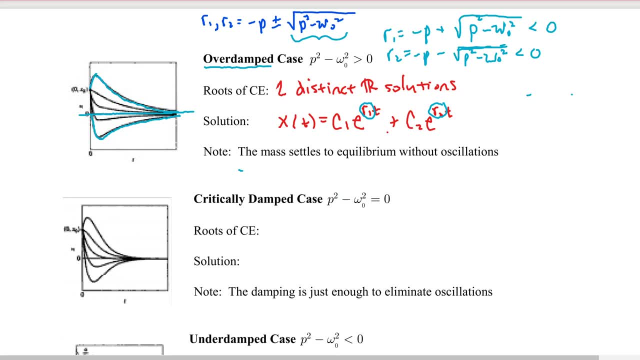 such that it's going to cause it to move slowly in either direction. So when we get two distinct real solutions of the characteristic equation, we have arrived at kind of an uninteresting overdamped case. The next case is called the critically damped case. 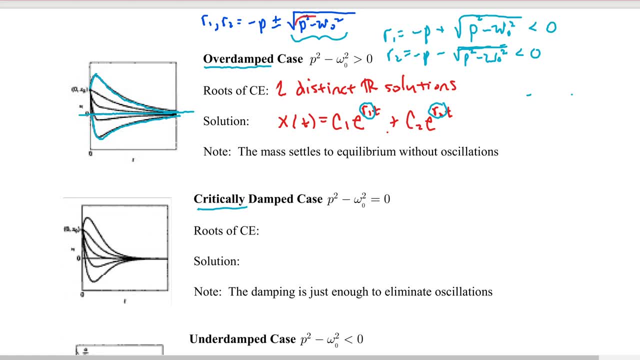 And this occurs when that important discriminant p squared minus omega- not squared- is equal to zero. Well, if that number is equal to zero, then the roots of the characteristic equation will simply be one repeated real solution, right? If this number over here is zero, negative p plus or minus zero is just negative p. 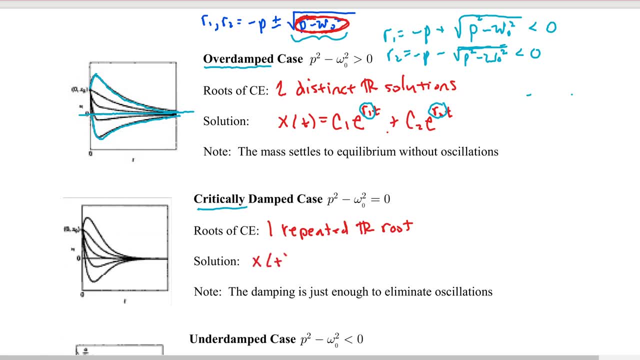 So the general solution then would look like: x of t equals e to the negative pt times c sub 1, plus c sub 2 times t. Or, if you want to see it expanded, that's c sub 1, e to the negative pt. 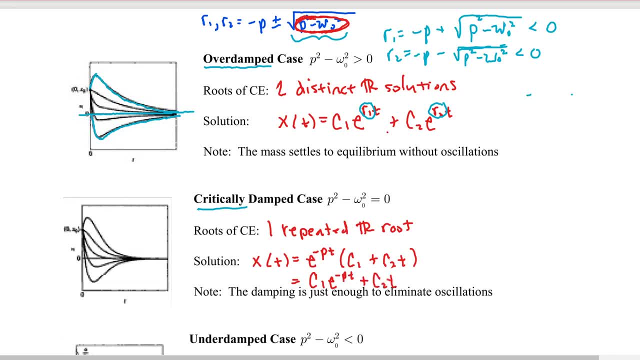 There's my x, That's the exponential term And, if you'll remember, we multiply the second one. We're dealing with multiplicity 2 here, so we need two terms. We multiply the second one by t in order to make those two terms linearly independent. 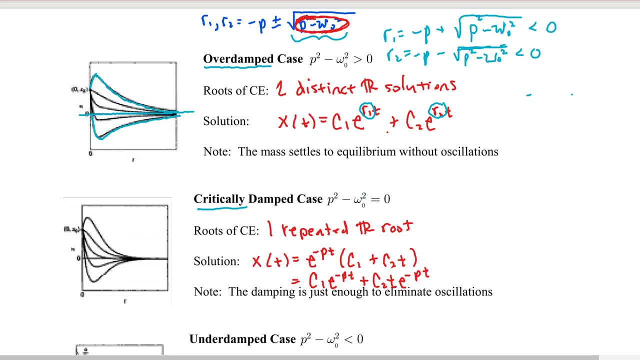 So in this case it's not overdamped. The damping is just enough to eliminate the oscillations. So, considering a couple of different initial conditions, if I toss the mass to the left it's going to settle pretty quickly back down to its equilibrium position. 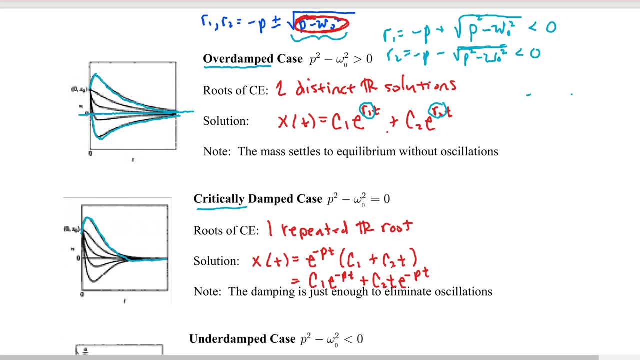 If I move a little faster than the overdamped case, so the resistance is not as strong, but it's not going to cross its equilibrium position. If I move it to the right and I toss it to the left, it's going to settle back down pretty freely to its equilibrium position. 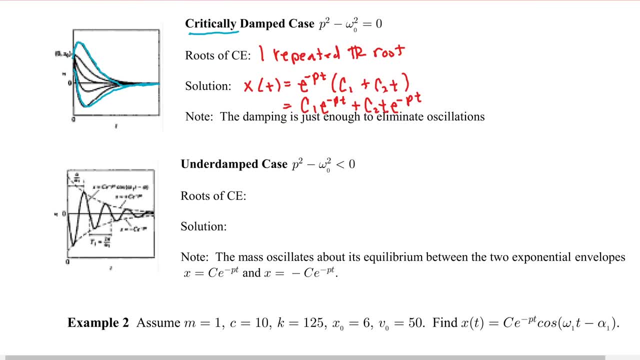 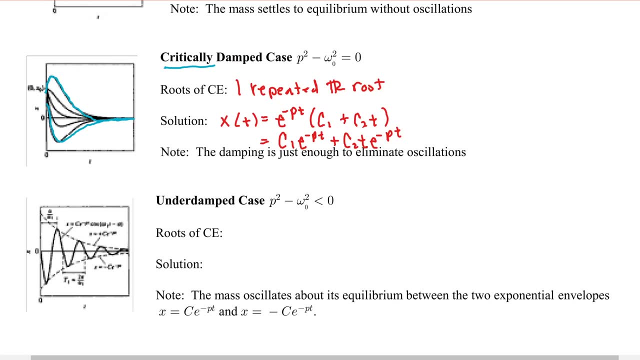 The last case, in my opinion, is the most interesting case. This is called the underdamped case. This will occur when our discriminant p squared minus omega, naught squared, is less than zero. Remember, if that discriminant is less than zero. 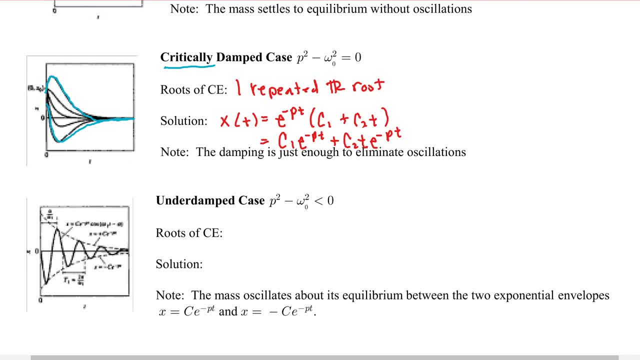 the square root of that number is an imaginary number. So we would end up with two complex roots of the form: negative, p plus or minus. Let's go ahead and factor out the i for the imaginary. If p squared minus omega naught squared is negative, then omega naught squared minus p squared is positive. 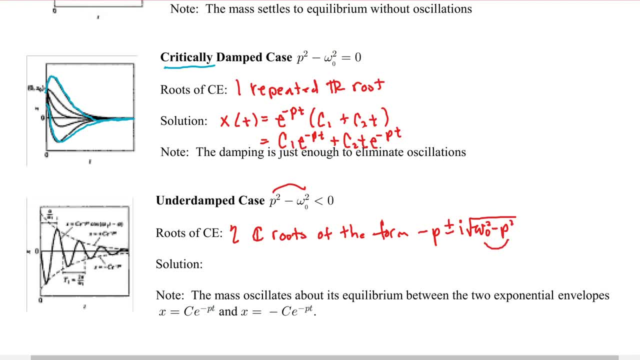 So by switching those two terms here in my discriminant I made that a positive number under the radical, but it's equivalent to the original because I extracted the i. So when we have two complex conjugate roots, the solution or the equation of motion, 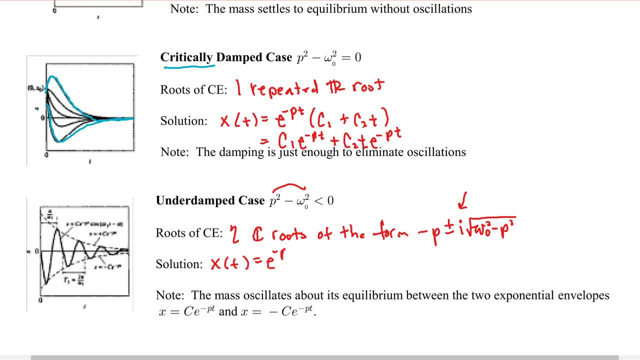 looks like e to the negative pt. I take the real part as the coefficient of t in the exponent times a cosine of. now I need this number as the coefficient of t in my cosine times a cosine of t in my cosine function. 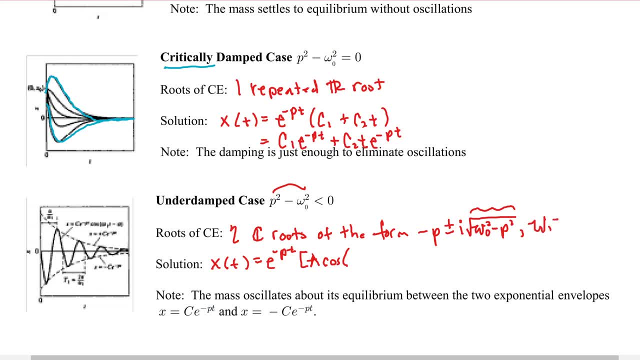 It's going to be a lot of details to write, so we're going to invent another constant. We'll call it omega one. Omega one will be square root of omega naught squared minus p squared, So that when we write our general solution here, 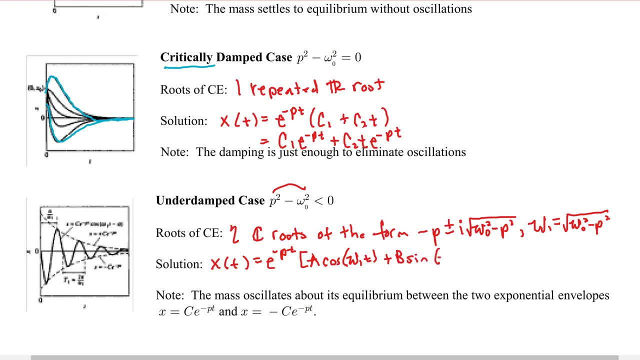 we can call this omega one t plus b sine of omega one t Or, as we saw in previous analysis, we'll be able to write this as a condensed cosine wave. So that's what we needed to c? e to the negative pt times: cosine of omega one t minus alpha. 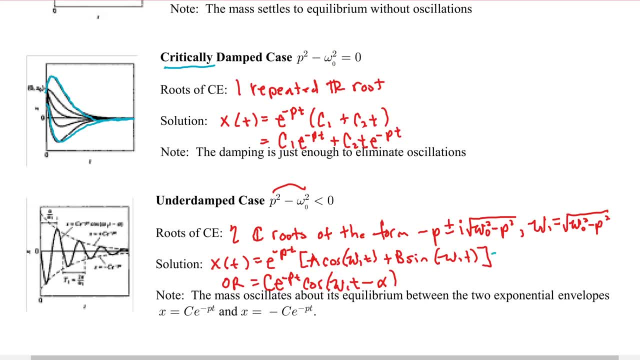 Now it's really beneficial in this case to condense from two trig functions to the single trig function, because now we can view this cosine wave as having an exponentially decreasing amplitude. Remember, the number to the left of cosine is your amplitude. Here we have a function. 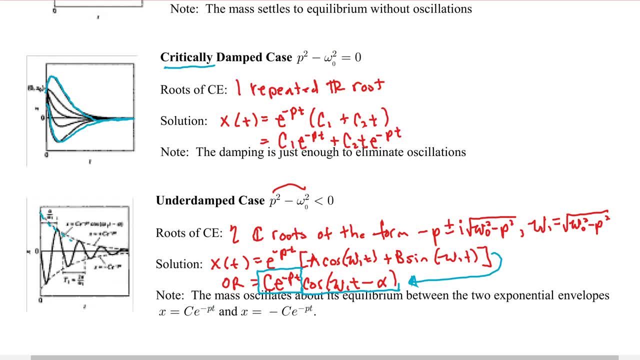 So c? e to the negative pt and negative c e to the negative pt create what we call two exponential envelopes, And the motion of the mass follows a cosine wave. But the cosine wave has an exponentially decreasing amplitude. So what happens to your mass is it oscillates. 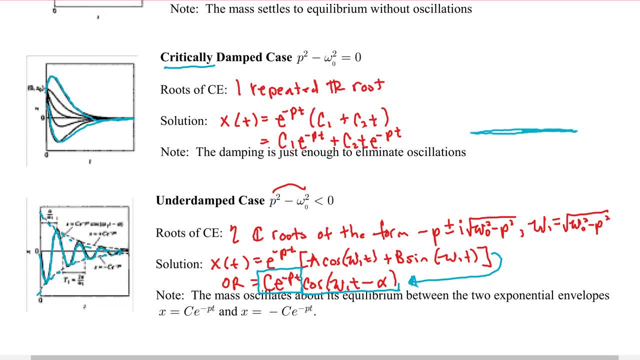 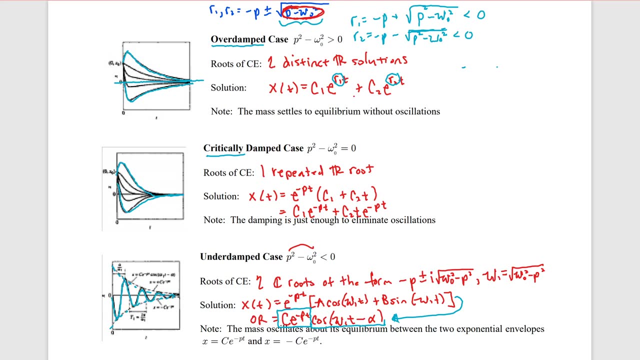 on either side of that equilibrium position, but each time it goes a little less far, until it settles down eventually in the center. So in summary here there are three possibilities for free damped motion, And each possibility is determined by the nature of the roots of the characteristic equation. 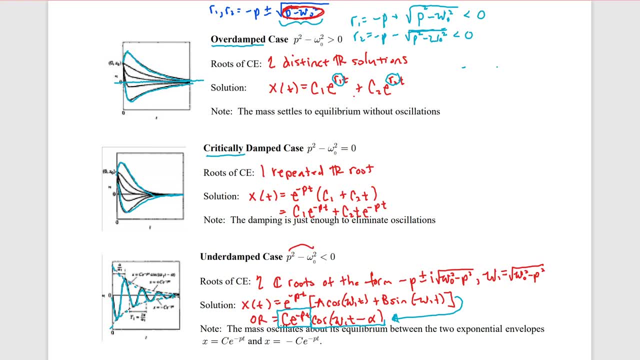 If our discriminant is positive, we end up with two distinct real solutions, yielding the overdamped case. If our discriminant is zero, we end up with one repeated real solution or the critically damped case. That is, there's just enough damping. 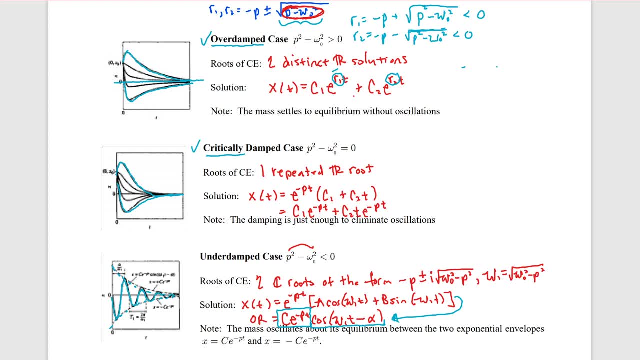 to eliminate the oscillations. And finally, if our discriminant is negative, we end up with two complex roots of the characteristic equation, yielding us to the most interesting underdamped case where the mass oscillates back and forth through its equilibrium position with an exponentially decreasing amplitude. 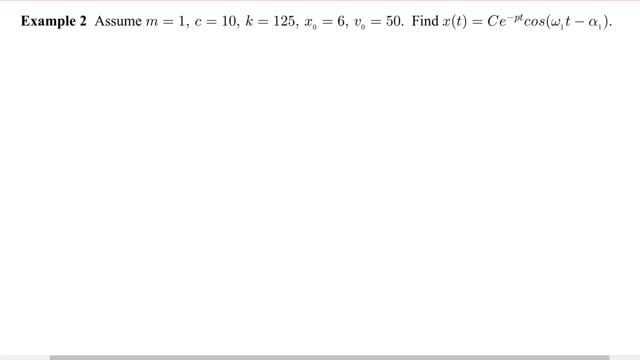 with each round of oscillation. So let's try an example of free damped motion. Assume the mass is 1, damping constant C is 10, spring constant K is 125, initial position X- naught is 6, initial velocity V- naught is 50. 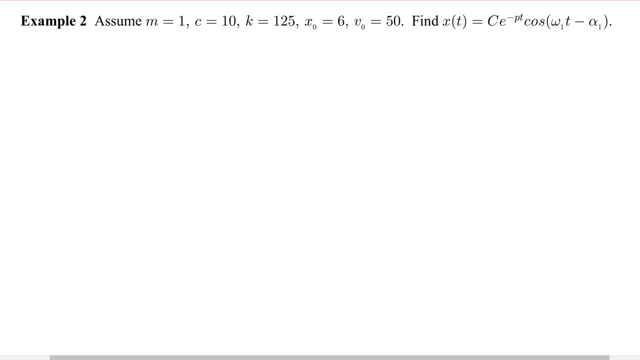 Find the solution X of T in the form CE to the negative P cosine, omega 1 T minus alpha 1.. So this one is very straight and to the point. We can go ahead and write our differential equation of motion without doing too much dimensional analysis. 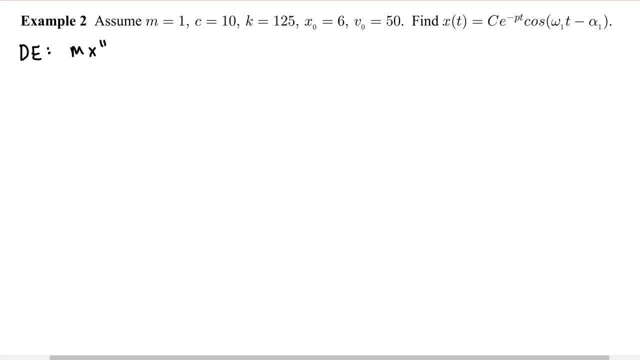 Our model is: MX double prime plus CX prime plus KX equals 0.. These constants are given directly, leading to the differential equation: 1X double prime plus 10X prime plus 125X equals 0.. The corresponding characteristic equation is therefore: R squared plus 10R plus 125 equals 0.. 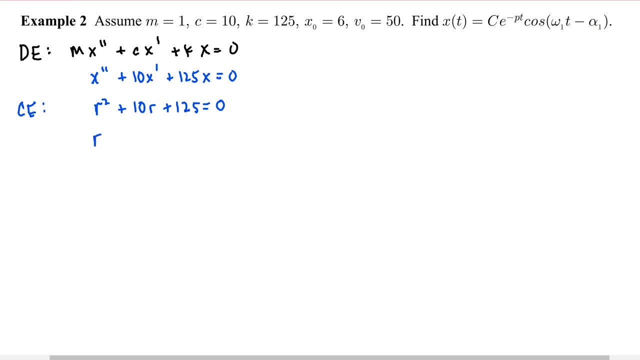 This quadratic does not factor, but we can outsmart it with the quadratic formula. We have negative B or negative 10, plus or minus the square root of B squared 10, squared minus 4 times A, which is 1, and C, which is 125. 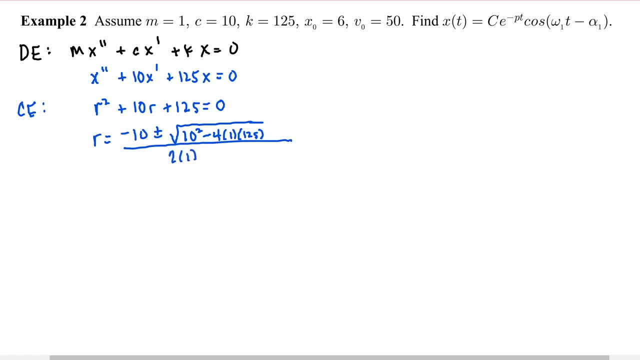 all divided by 2 times A or 2 times 1.. Simplifying, we obtain negative 10 plus or minus the square root. 10 squared is 100.. 4 times 125 is 500.. So we have 100 minus 500. 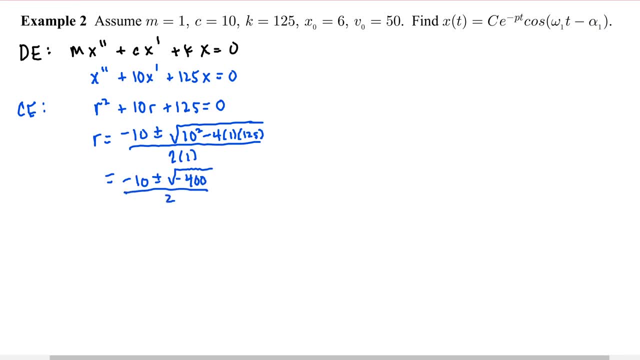 or negative 400, all divided by 2.. Let's simplify our square root as plus or minus 20I and divide both parts by 2.. We end up with negative 5, plus or minus 10I, Since we have two complex conjugate solutions. 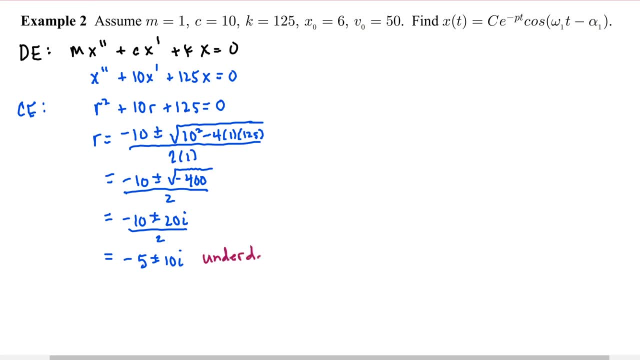 this is the underdamped case. Of course, I'm going to pick this one because this one's the most interesting. So, based on the nature of the roots of our characteristic equation, we can write our general solution We're going to end up with 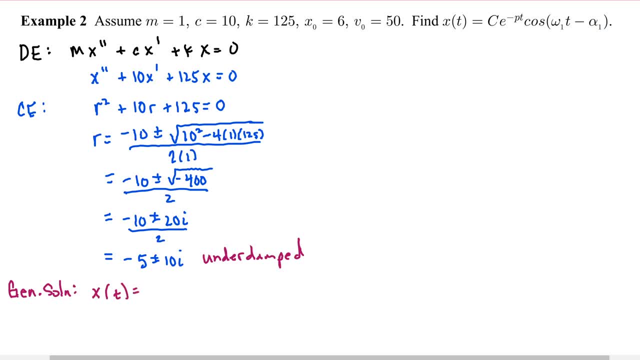 position. function X of T equal to E to the negative. Now remember we put the real part here as the coefficient on T. Notice, this exponential term does not need an arbitrary coefficient. Sometimes we like to put the arbitrary constant here. but save your two arbitrary constants. 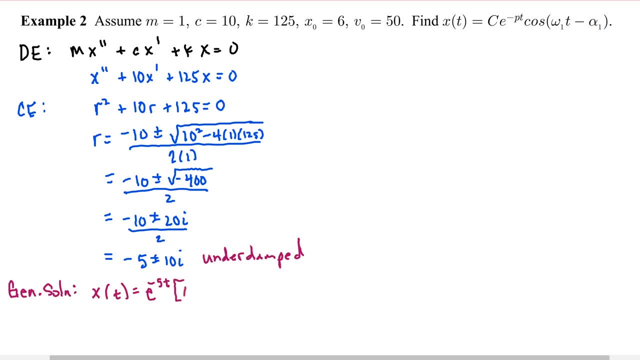 to go with your sine and cosine terms. So we have A sine of 10T. Actually, since in our triangle our A went with cosine, let's do A cosine 10T plus B sine of 10T. That way all of our notation will be consistent. 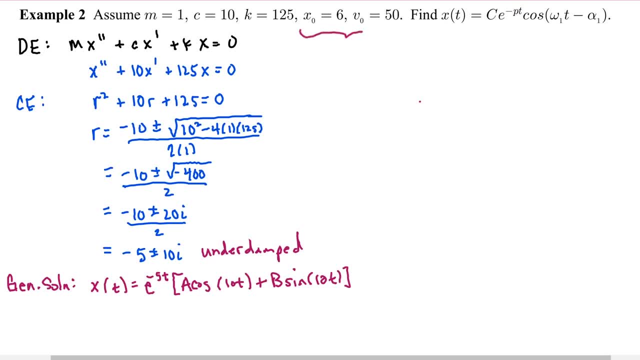 Now we do have a couple of initial conditions. One is for initial position, the other one's initial velocity. So at this time, I'm going to take the opportunity to find X prime of T. We will have to apply the product rule, since we're dealing with two. 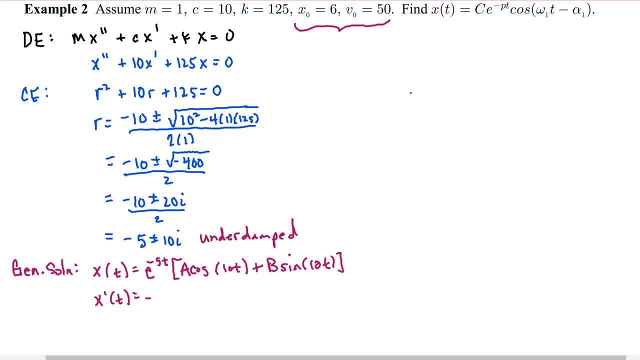 the product of two functions of T. So our first function is E to the negative 5T and we'll multiply by the derivative of the second function. That's going to give me negative 10A sine of 10T plus 10B cosine of 10T. 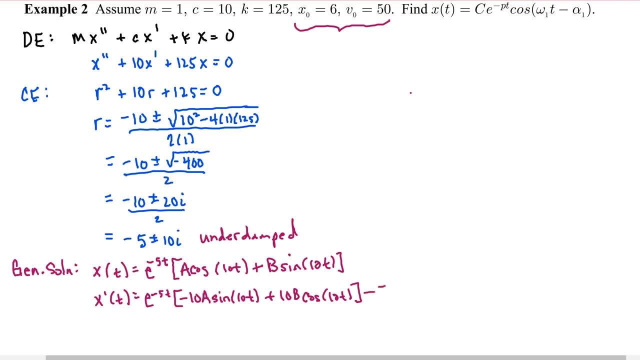 Okay, Plus the derivative of the first function, that's going to be negative 5E to the negative 5T times the second function, as is A cosine of 10T plus B sine of 10T, Looking at the given initial conditions. 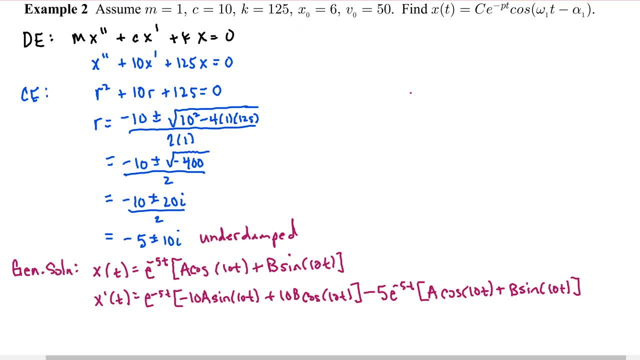 they're expressed maybe in a different format than we've used before. We have: X naught equals 6.. This is equivalent to saying the position at time 0 is equal to 6. And here the velocity at time 0 is equal to 50,. 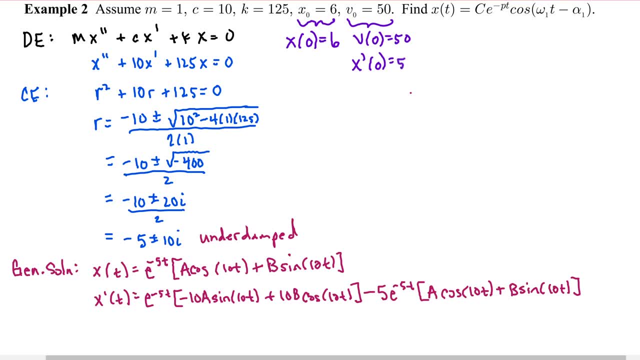 which we know is equivalent to X. prime of 0 equals 50.. So let's take those initial conditions and apply them to our general solution. X of 0 equals 6 is our initial position And X prime of 0 equals 50. 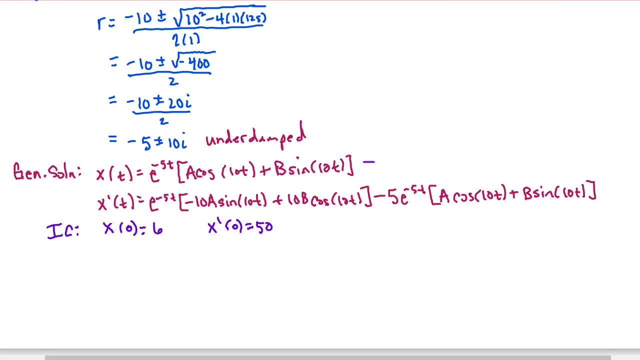 is our initial velocity. I'm just going to eyeball this here and not show too much work, But we want to go to our position- function X of T- and we're going to plug 0 in for T. Notice when we plug 0 in. 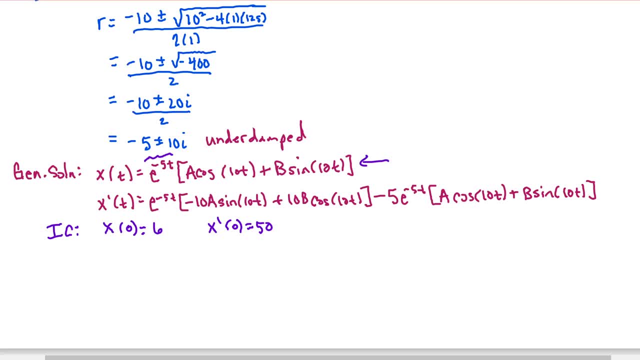 to our exponential term, E to the 0th power is just 1.. When we plug 0 in for cosine, we're going to get 1. And when we plug 0 in for sine, that whole term goes away. So very easily. 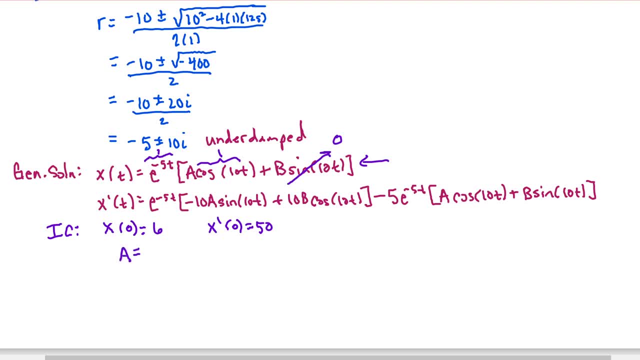 when we set this function equal to 6, we can see that A equals 6.. Let's do the same thing with X prime of 0.. X prime of 0 is equal to 50.. When we plug 0 in here, 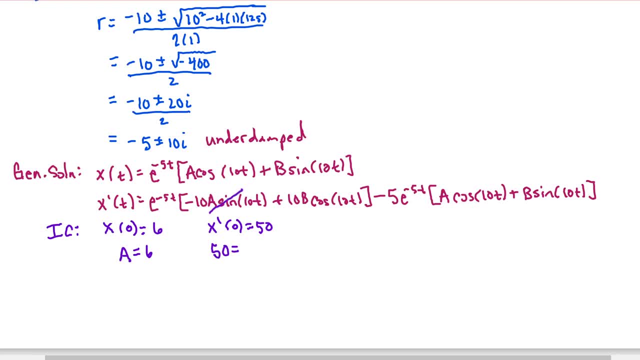 we get 1.. Sine of 0 is 0. And 10B times cosine of 0, that gives us 10B Working here. since E to the 0th is 1, we have minus 5.. 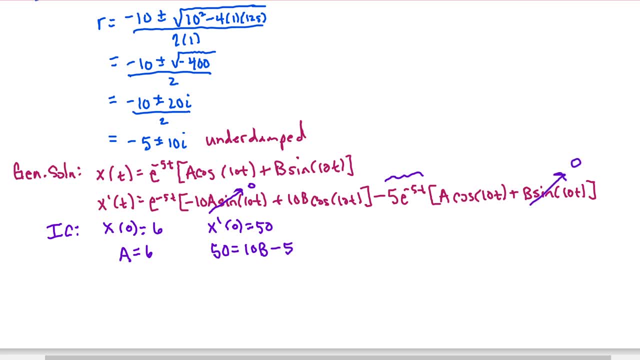 Recall: the sine of 0 is 0. And A times cosine of 0,, that's A times 1.. So we end up with this equation. Now we already know that A equals 6.. So I'm going to plug that in. 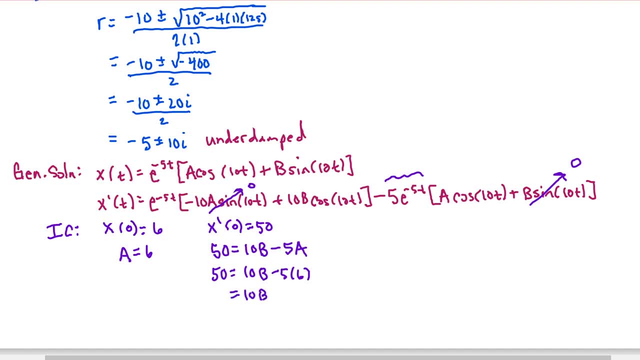 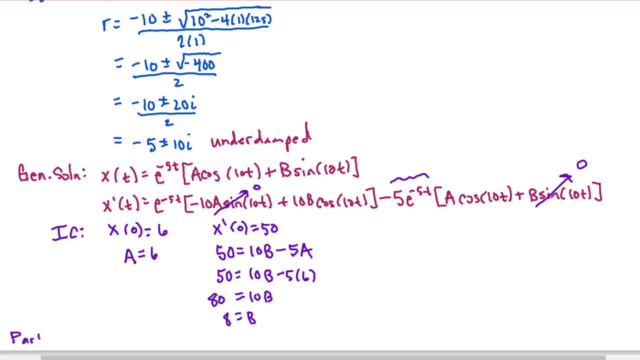 and see if we can solve for B here. Looks like very easily. B is equal to 8.. Therefore, our particular solution is: X of t equals E to the negative 5t times A, which is 6, cosine of 10t. 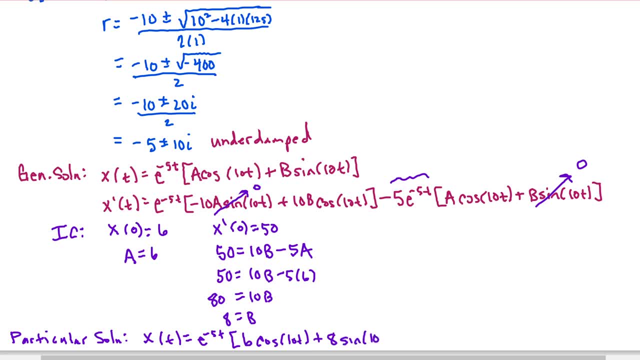 plus B, which is 8, sine of 10t. So that's the initial form of our particular solution, but we are going to condense it just a little bit, Making convenient use of a right triangle and Pythagorean theorem. 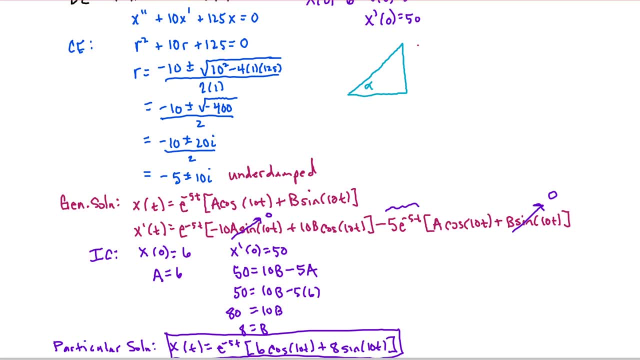 we're going to label the horizontal segment of this triangle whatever the coefficient of cosine is. In this case it's 6.. The vertical segment will be 8.. We can solve for the hypotenuse: 6 squared is 36.. 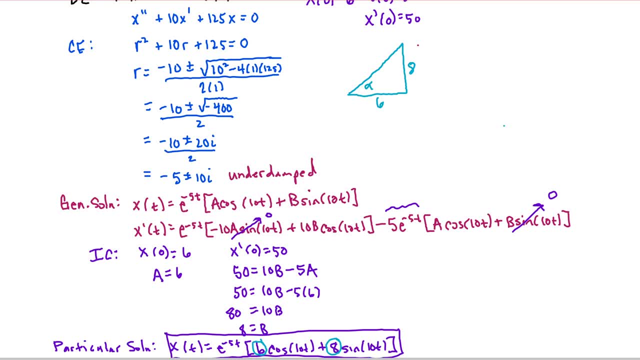 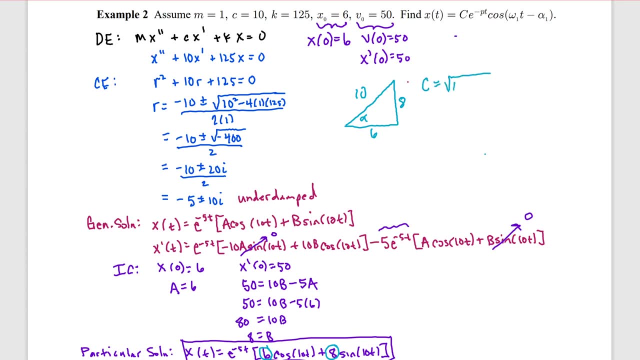 8, squared is 64.. Add those together to get 100.. And the square root of 100 is 10.. So, to be very clear, the amplitude given by C in this case is 10.. So we have found this constant right here. 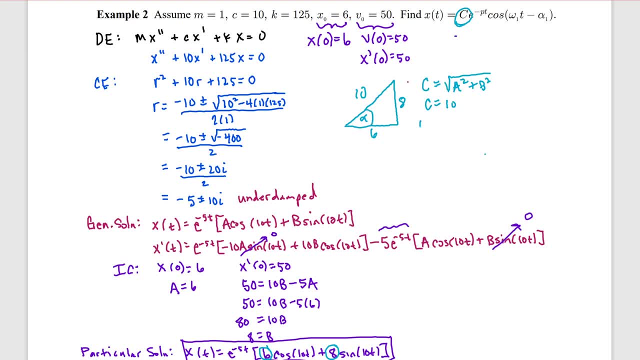 Let's go ahead and use this right triangle to figure out alpha. We can use inverse tangent of Y divided by X or B divided by A and approximate this with our calculator. in radians We get about 0.9273.. Thus our condensed particular solution. 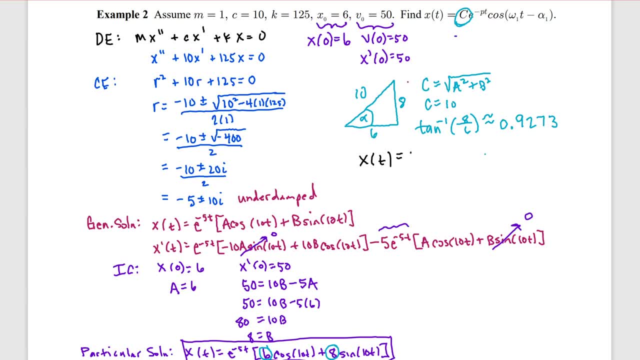 will be: X of t equals amplitude 10, our exponential part e to the negative 5t times cosine of 10t minus alpha 0.9273.. So the mass will oscillate to the left and to the right according to this cosine wave. 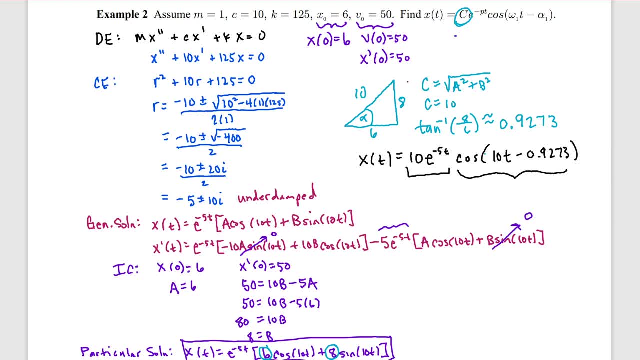 but it's going to have an exponentially decreasing amplitude. So the way that we can think about this, if we imagine the graph- or you can certainly use your calculator to sketch the graph- we're going to have two exponentially decreasing curves Or one decreasing 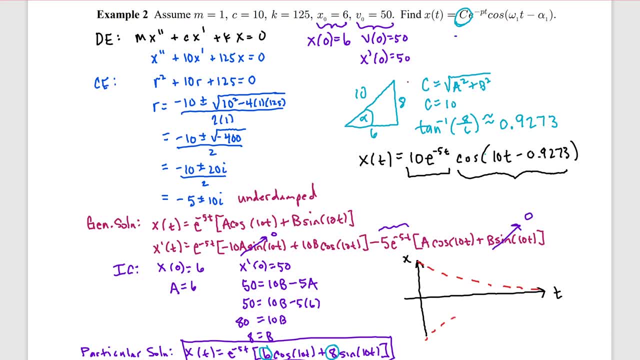 and one- the mirror image here coming up from the bottom. So the first exponential envelope would be 10e to the negative 5t and the other one, the mirror image, negative 10e to the negative 5t. Our initial position was: 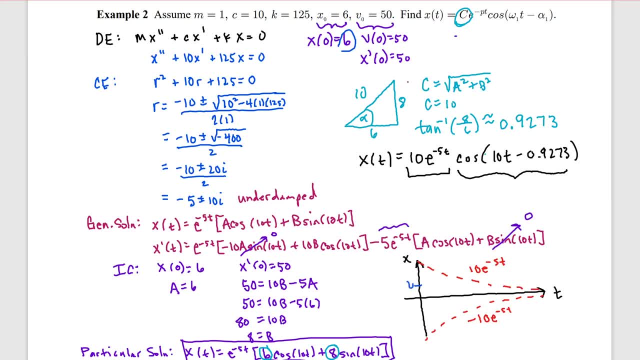 positive 6. And the initial velocity was also positive. so it's going to begin moving to the right And then it's going to follow a cosine wave with an exponentially decreasing amplitude If we manipulate this function just a little bit further, that is, I'm going to factor the 10 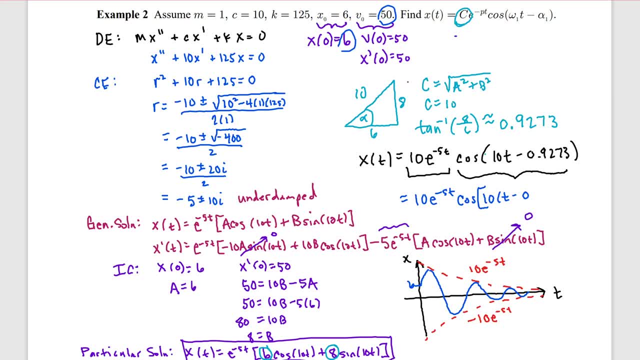 out of the argument, changing this number to 0.09273, just by factoring out the 10. Then the lag time is given by this very small number. right here Also, we have something called a pseudo-period Running out of space here. 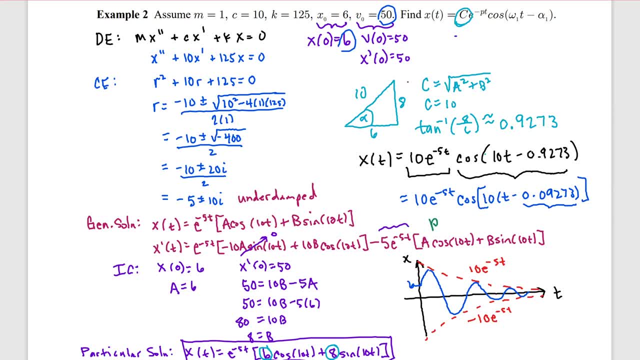 Let's see I'm going to fit it right in right here, The pseudo-period, false period. we're going to find the period like normal: 2pi over 10, or pi over 5.. This is going to tell me. 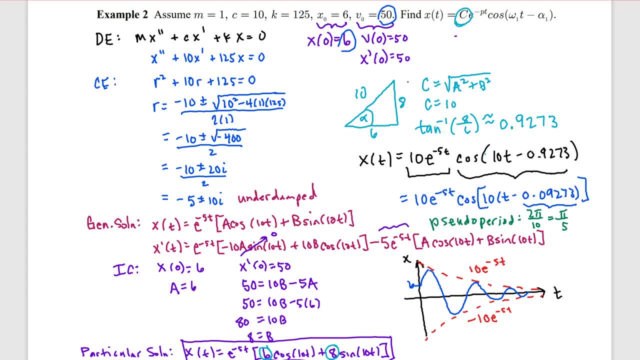 the length that I get sort of a cosine wave, a fundamental cosine wave. So what's going to happen? we've got a little bit of lag time here, So not drawn to scale, obviously, But this distance right here is our lag time. 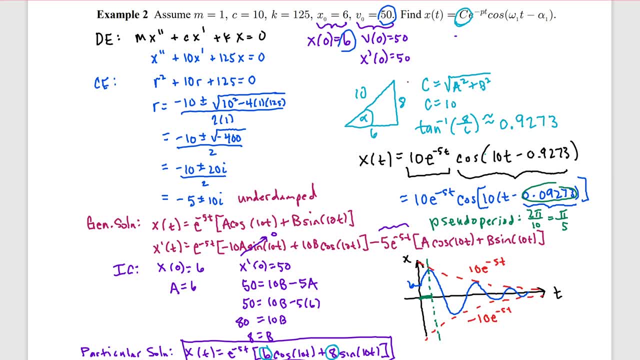 Think of it as a horizontal shift And then, from the top of my cosine wave to what would be the top of the other side, although my amplitude is exponentially decreasing. what we have right here, this distance, is our pseudo-period pi over 5.. 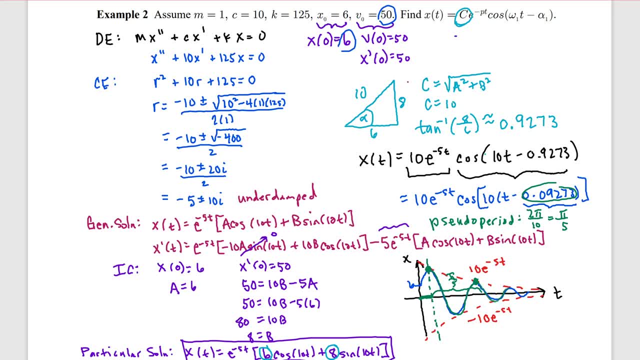 And then, according to the next fundamental cycle of cosine, that bowl shape, we get another distance of pi over 5.. So the mass is going to oscillate on either side of its equilibrium, but each time it's going to have a smaller and smaller amplitude. 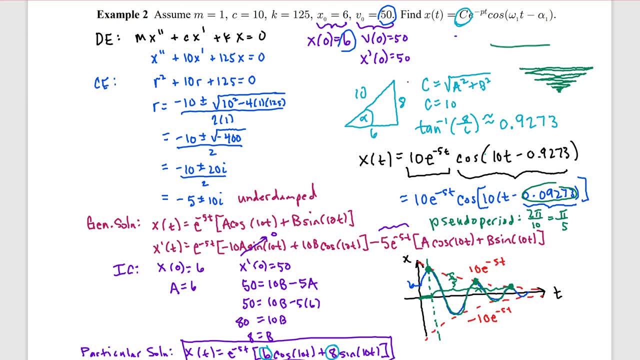 until it sort of settles down in the middle. And of course this happens on one dimension. but I was moving down so you can kind of see how I'm moving the mass. Remember, whenever the position is to the right, x is positive. 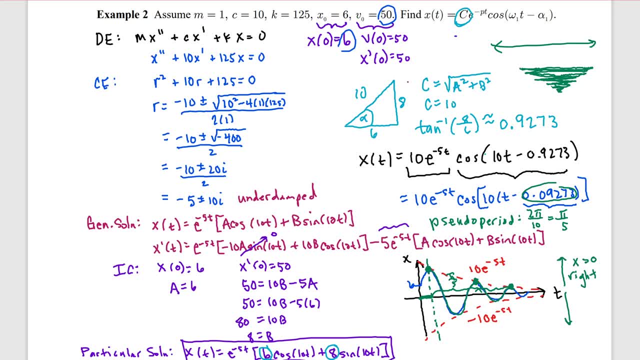 x in this case is our vertical axis and when x is negative, position is to the left. So this is a classic underdamped case, A free damped motion. So we have taken a very simple differential equation: linear, homogeneous differential equation. 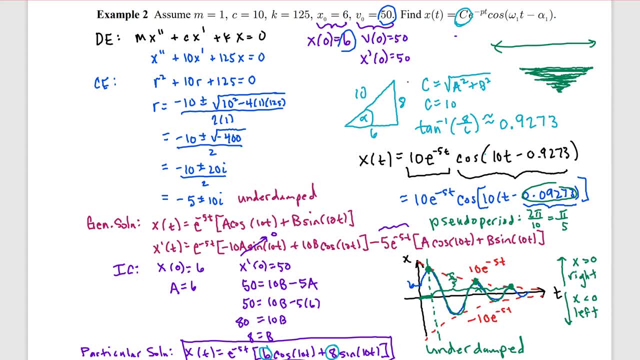 with constant coefficients that we can solve very efficiently and quickly with a characteristic equation, and we've applied it to a simple harmonic oscillator, both with free undamped motion and now examining free damped motion, So that differential equation creates a very useful model. with lots of mechanical vibrations. 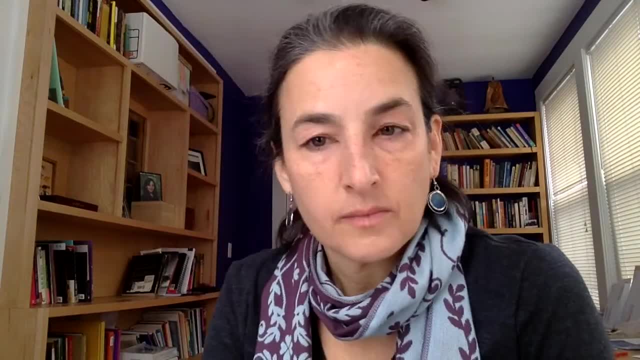 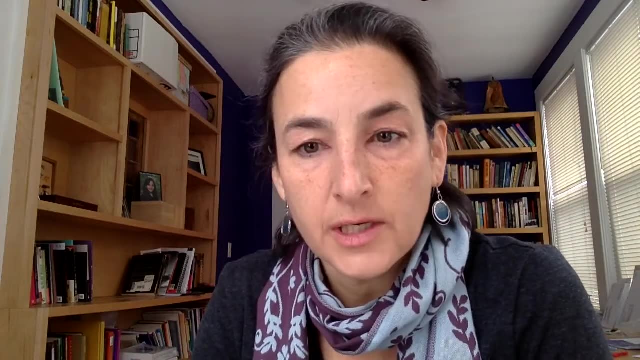 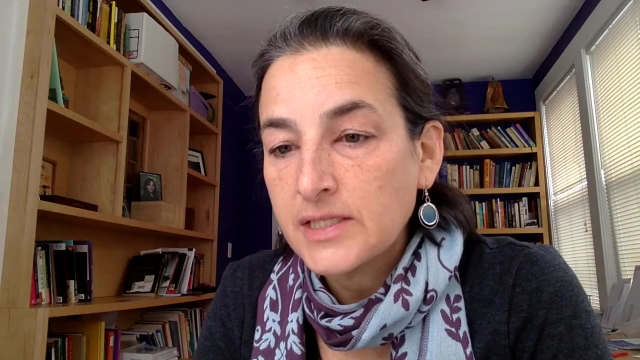 Hi, I'm Beth Rubin. I am an associate professor of education at Rutgers, the State University of New Jersey in the United States, And in my research I look at how young people come to see themselves as citizens, And I look at this across a variety of settings, taking into account